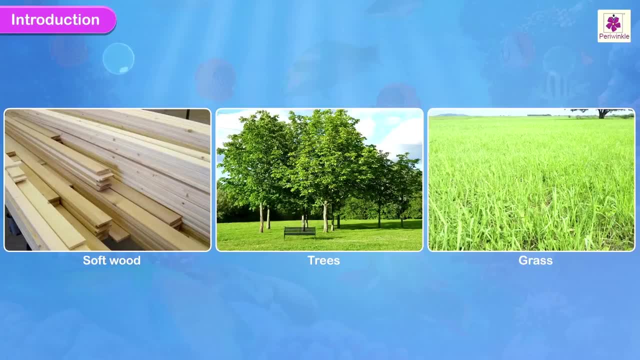 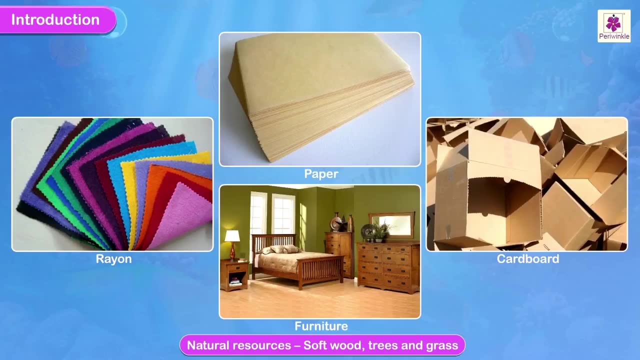 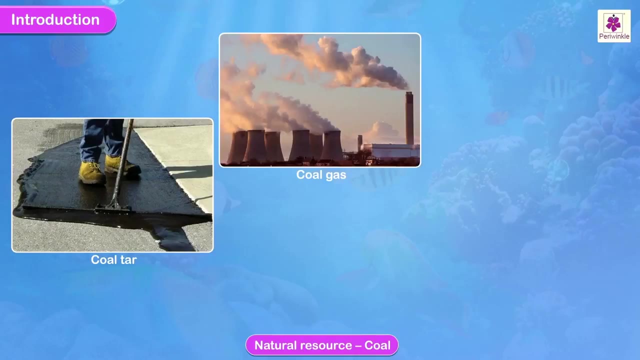 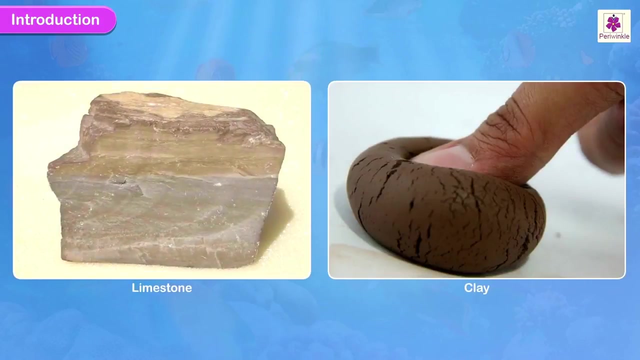 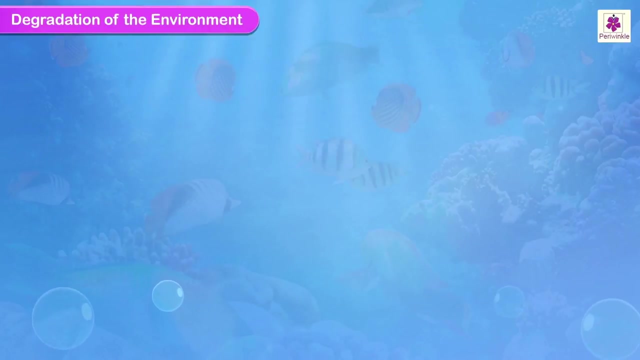 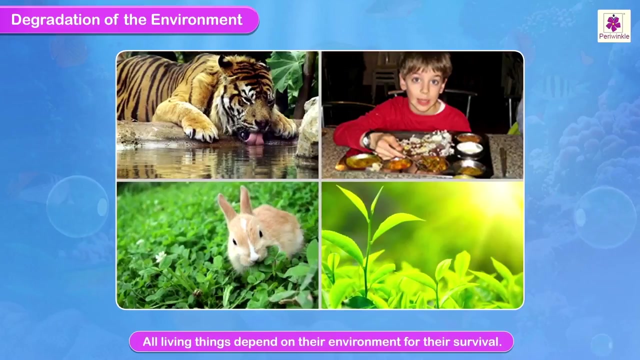 They are used for man-made products like rayon, paper, cardboard, furniture, etc. Coal is the natural resource for coal, tar, coal, gas, dyes, coke, etc. Limestone and clay are the raw materials for Portland, cement, concrete, etc. All living things depend on their environment for their survival. 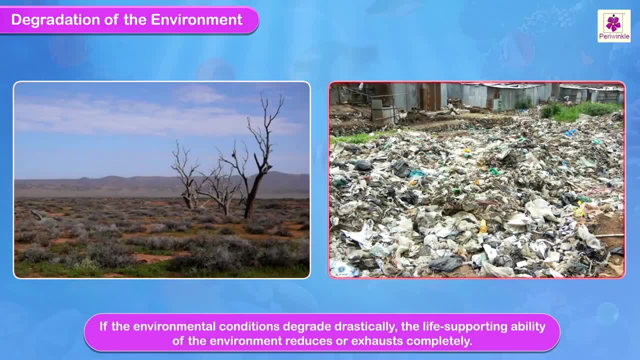 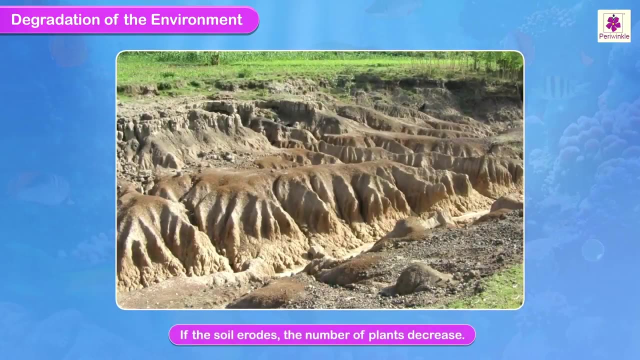 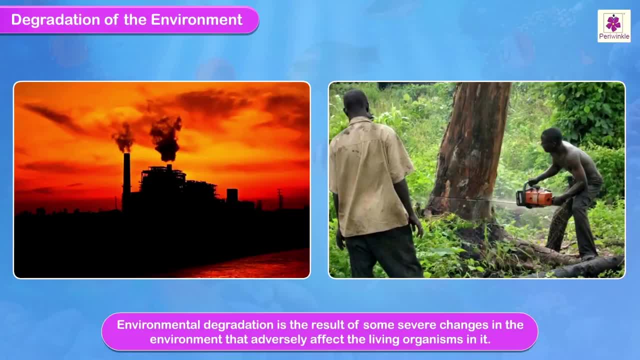 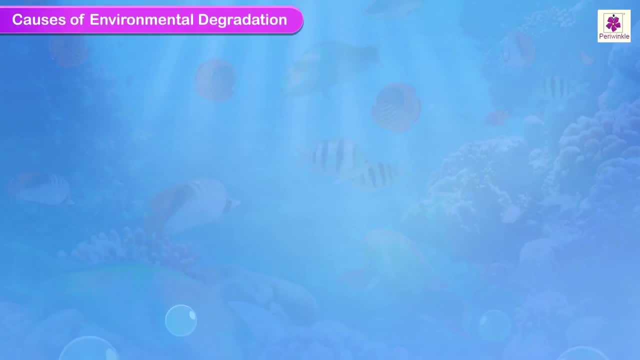 Toilet flush is the result of some severe changes in the environment that adversely affect the living organisms in it. Causes of Environmental Degradation, Natural Causes, Floods, earthquakes, tsunamis and volcanic eruptions are some of the natural causes that degrade the environment. 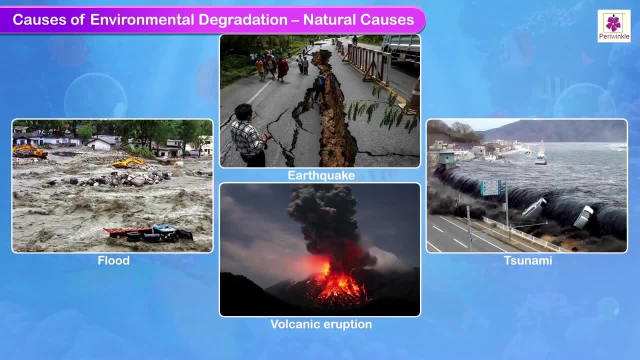 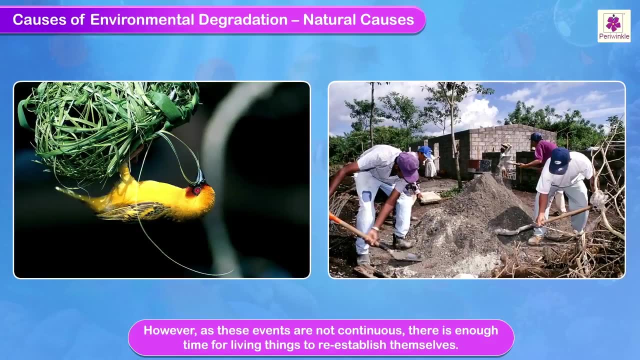 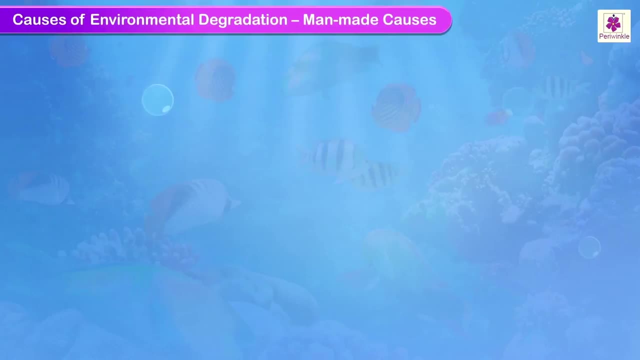 Natural Causes: Floods, earthquakes, tsunamis and volcanic eruptions are some of the natural causes that degrade the environment. Natural Causes. However, as these events are not continuous, there is enough time for living things to re-establish themselves. Manmade Causes. 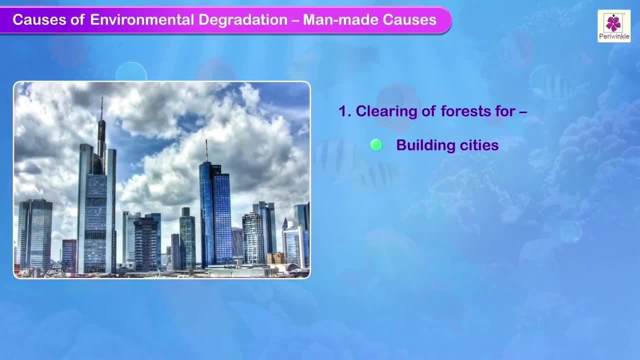 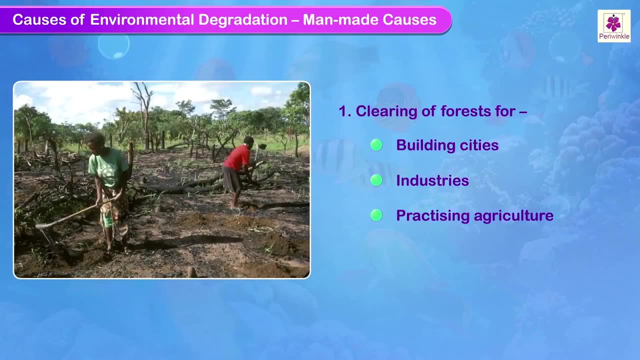 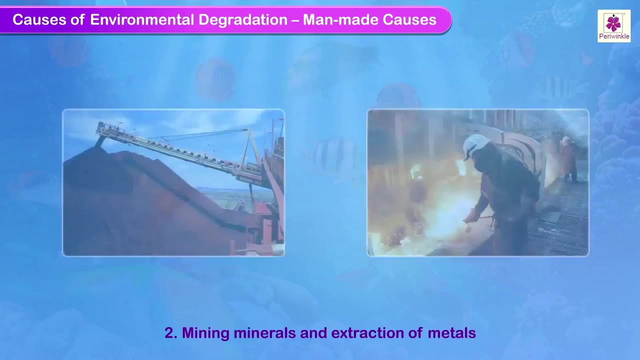 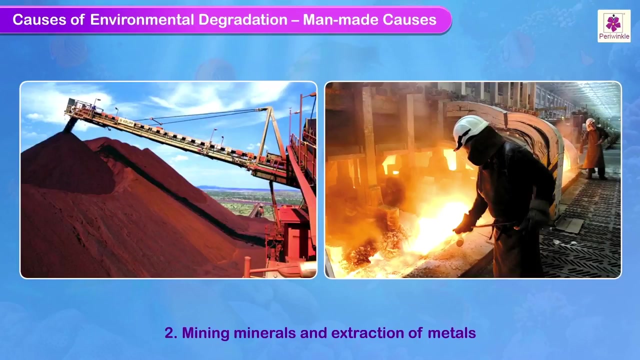 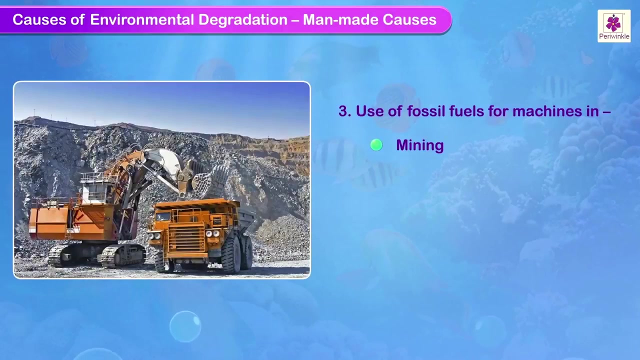 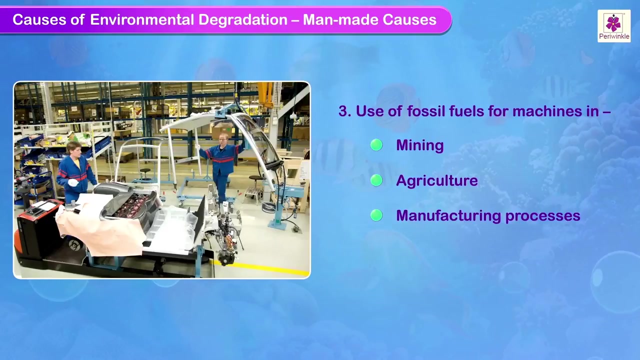 Clearing of forests for building cities, industries, practicing agriculture and extracting natural resources, mining minerals and extraction of metals for use in industries. use of fossil fuels for machines required for mining, agriculture, manufacturing processes and transport. use of. 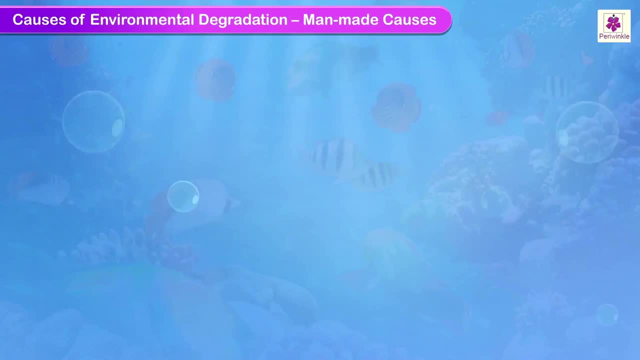 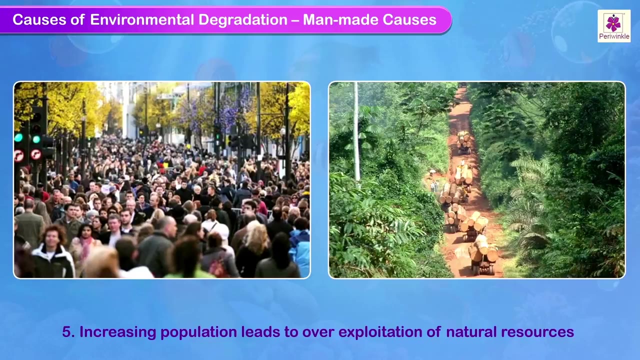 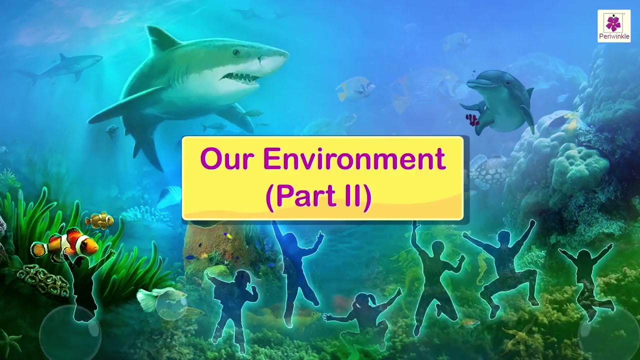 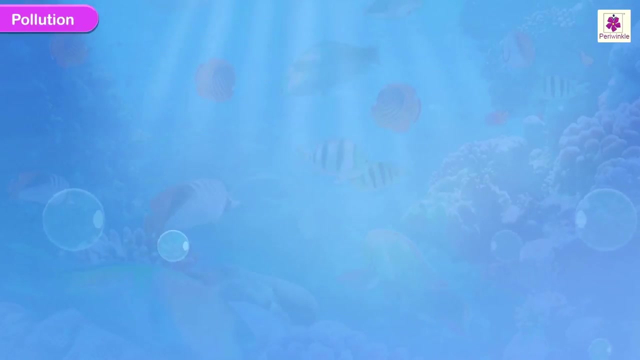 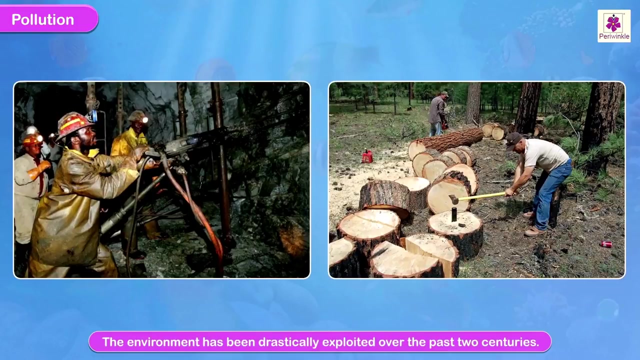 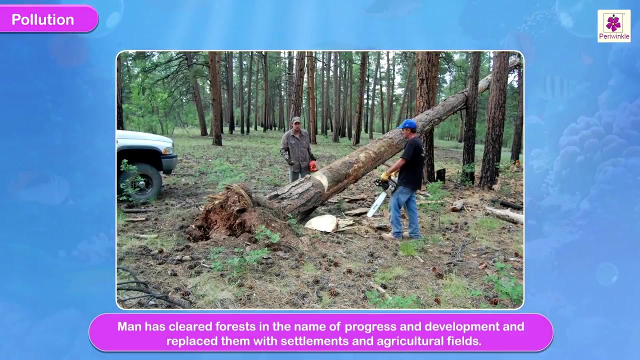 fertilizers and pesticides. Increasing population leads to over-exploitation of natural resources, Our Environment, Consequences of Environmental Degradation, Pollution. The environment has been drastically exploited over the past two centuries. Man has cleared forests in the name of progress and development. 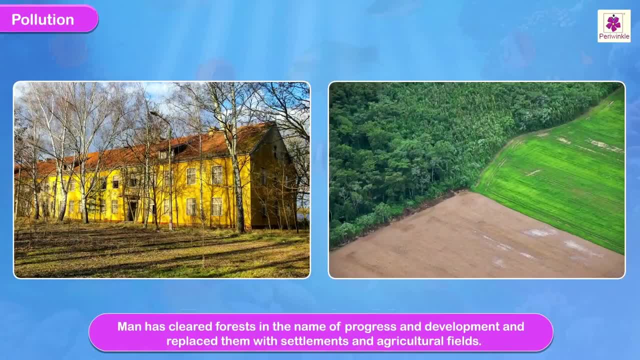 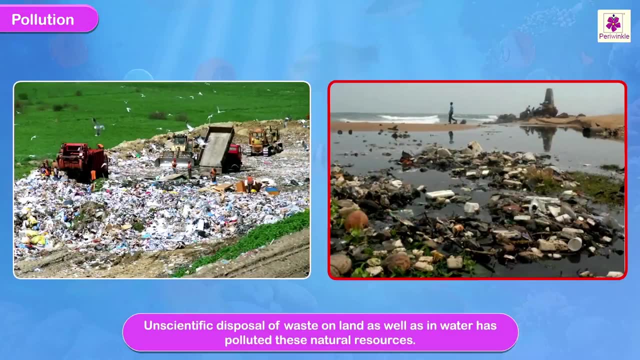 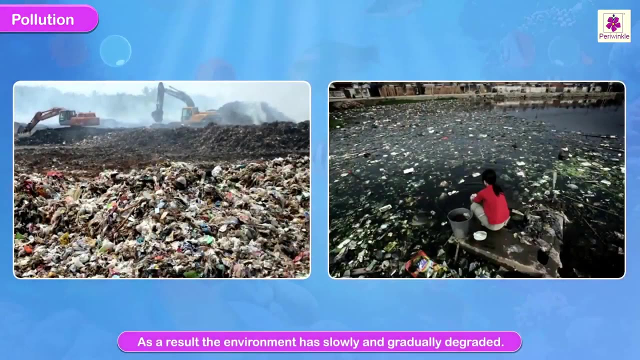 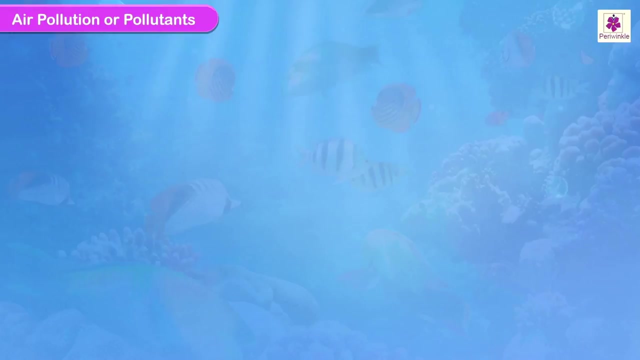 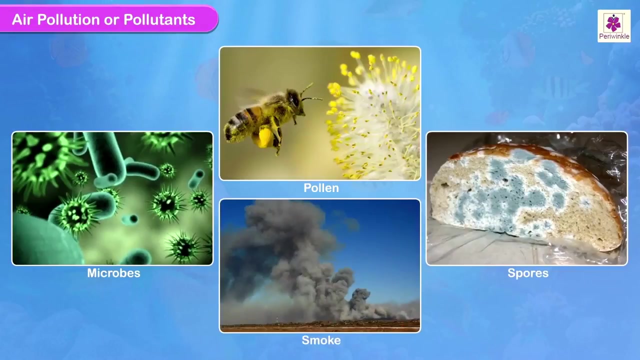 and replaced them with settlements and agricultural fields. Unscientific disposal of waste on land, as well as in water, has polluted these natural resources. As a result, the environment has slowly and gradually degraded Air Pollution, or Pollutants: Microbes, pollen, spores, smoke, dust, fiber. 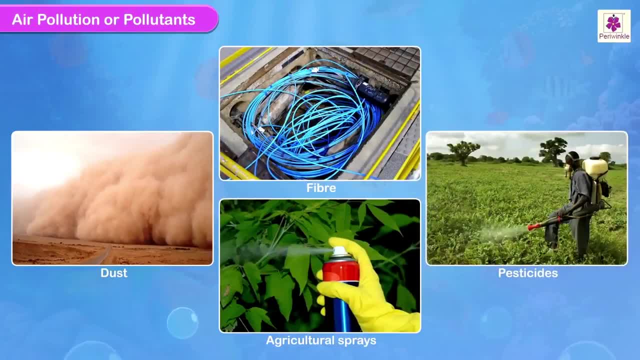 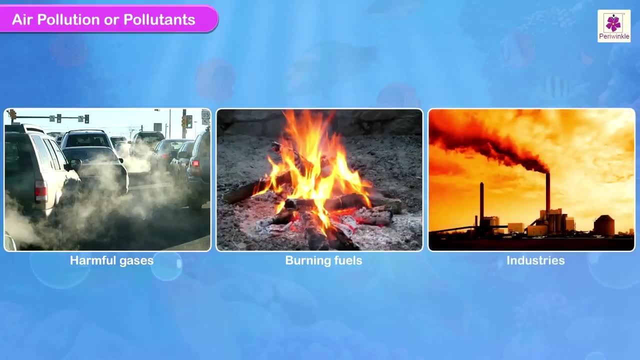 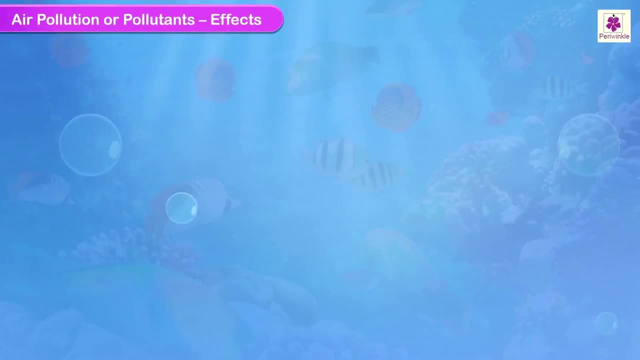 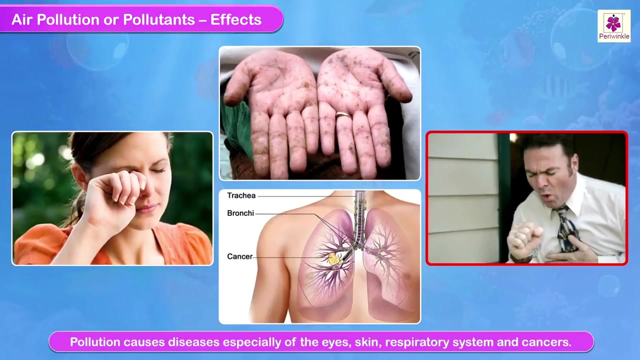 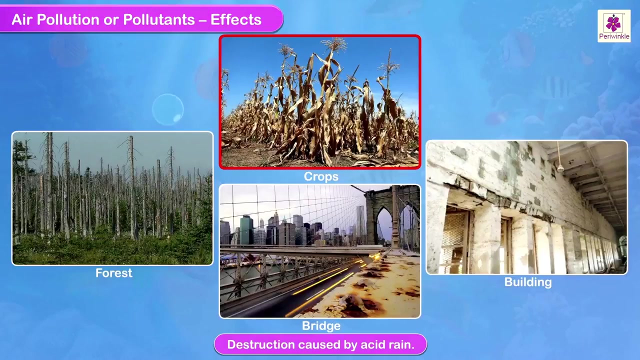 pesticides and other agricultural sprays. Harmful gases given out by automobiles, burning fuels and industries are some air pollutants Effects. Pollution causes diseases, especially of the eyes, skin, respiratory system and cancers. Acid rain destroys forests, crops, buildings. 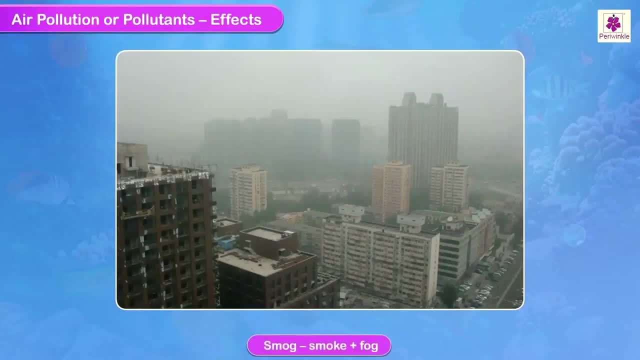 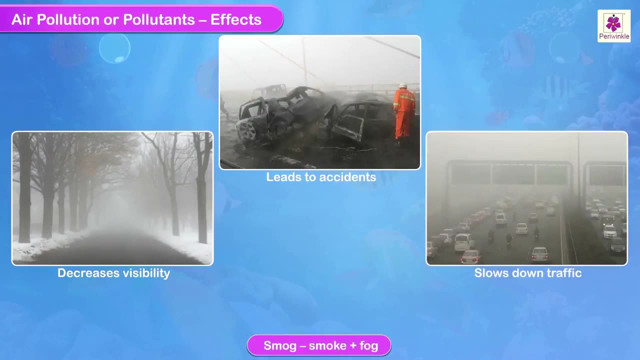 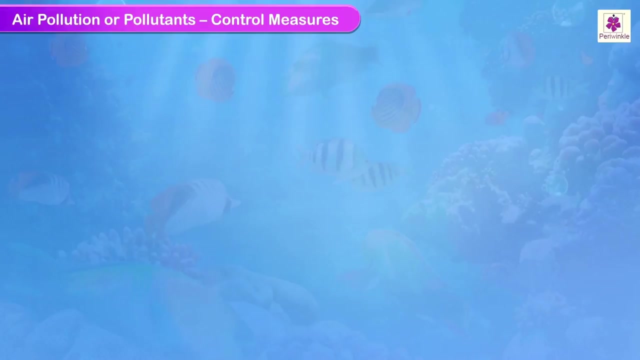 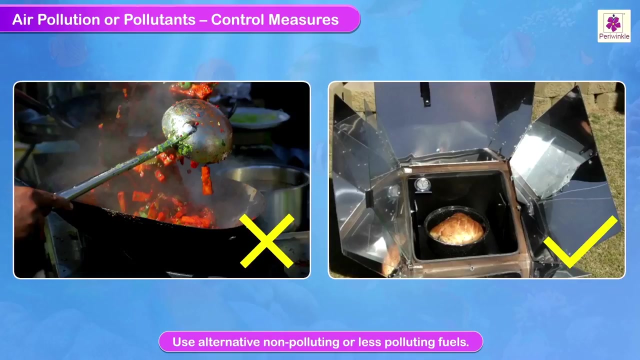 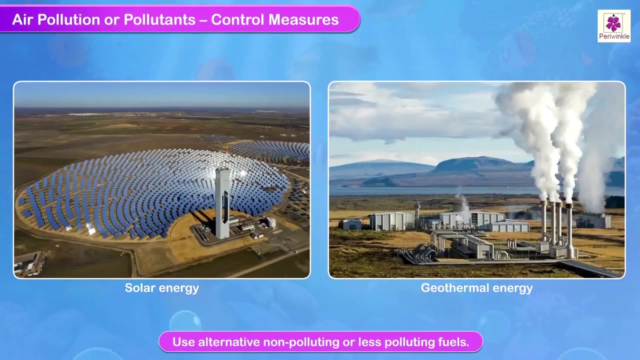 and bridges. Smog, ie smoke plus fog, decreases visibility, leads to accidents, slows down traffic and delays flights. Control Measures: Use alternative, non-polluting or less-polluting fuels, eg. solar energy, geothermal energy, etc. 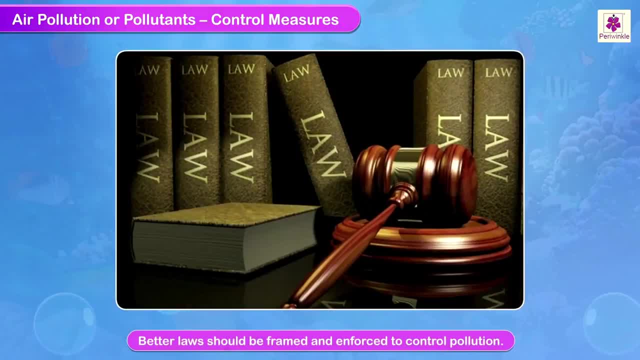 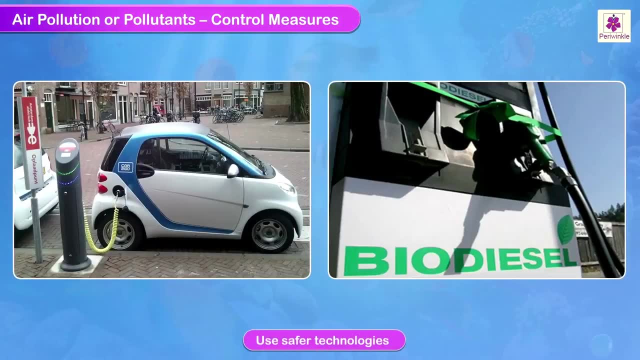 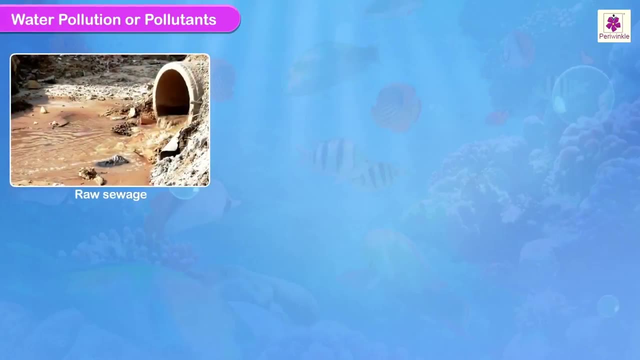 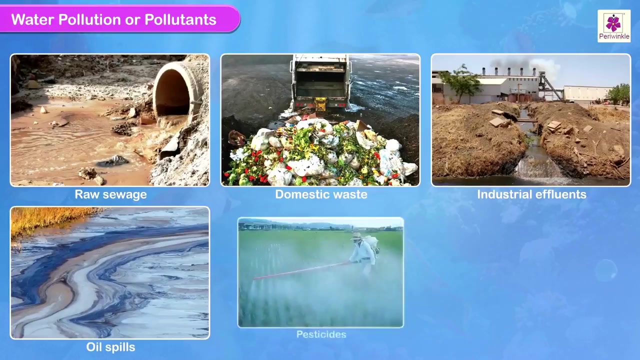 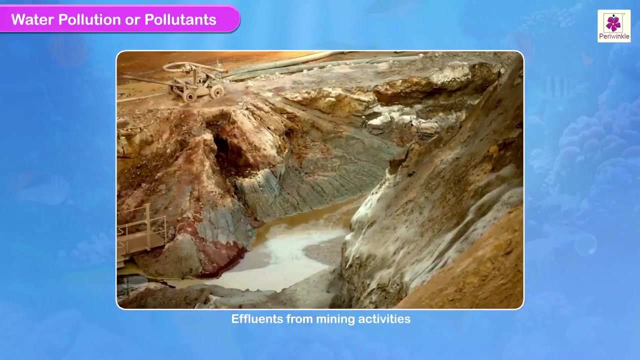 Better laws should be framed and enforced to control pollution. Use safer technologies. Water Pollution or Pollutants, Raw sewage, domestic waste, industrial effluents, oil spills, pesticides, fertilizers and effluents. Effluents from mining activities are common water pollutants. 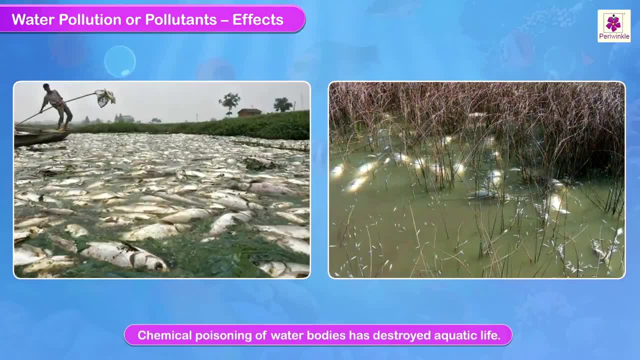 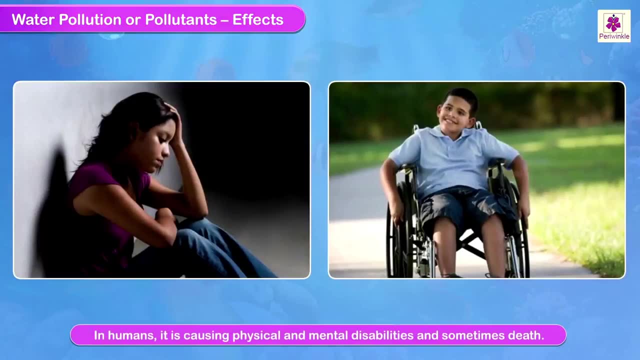 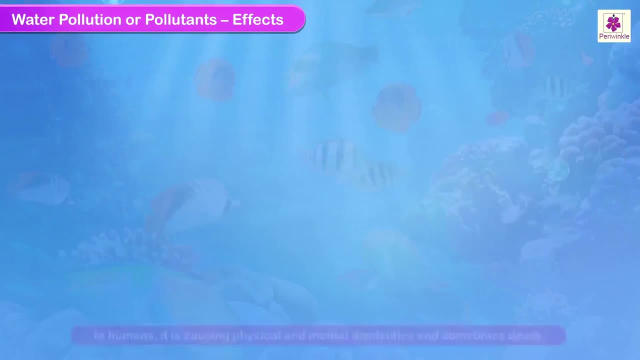 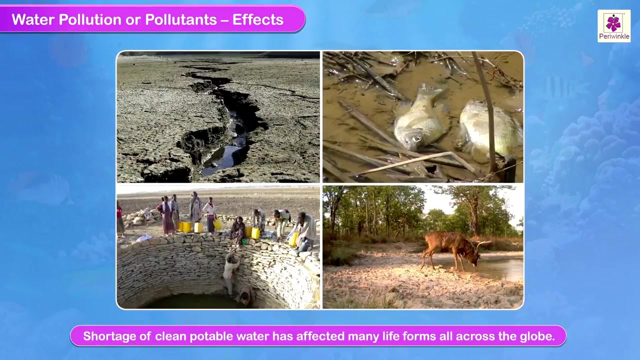 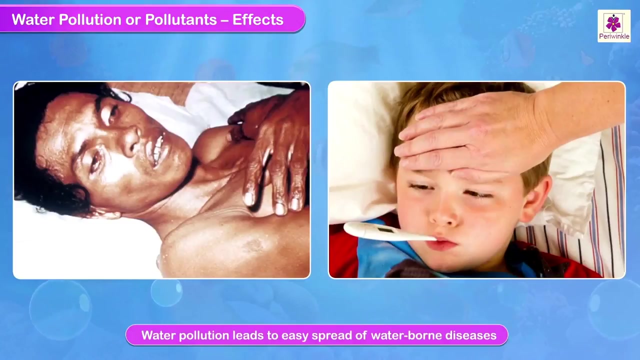 Effects. Chemical poisoning of water bodies has destroyed aquatic life In humans. it is causing physical and mental disabilities and sometimes death. Shortage of clean potable water has affected many life forms all across the world. Water pollution leads to the easy spread of water bone diseases. 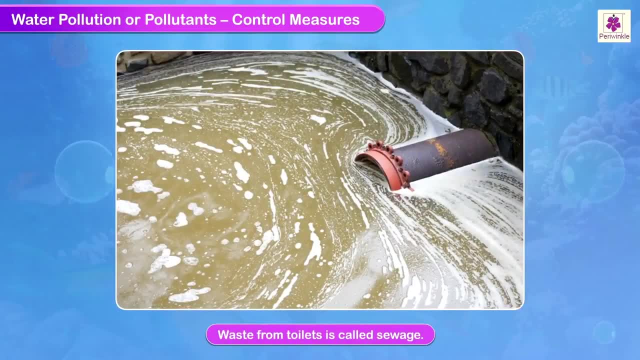 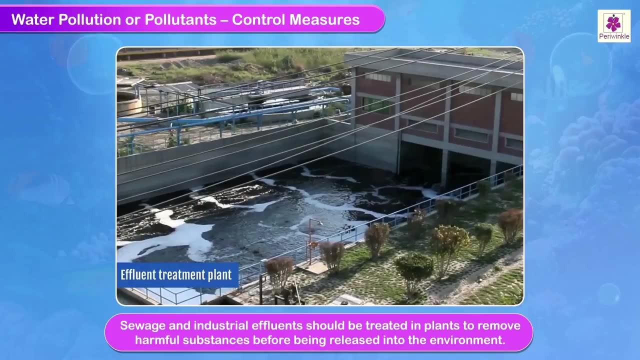 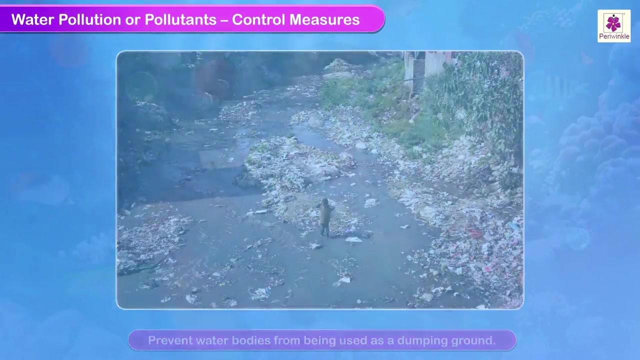 Control Measures. Waste from toilets is called sewage. Sewage and industrial effluents should be treated in plants to remove harmful substances before being released into the environment. Prevent water bodies from being used as a dumping ground. Make less use of chemical fertilizers and pesticides. 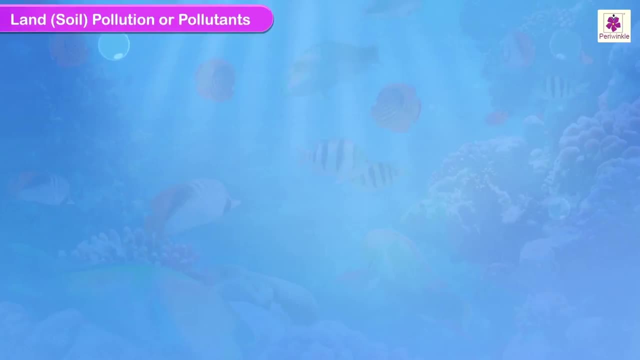 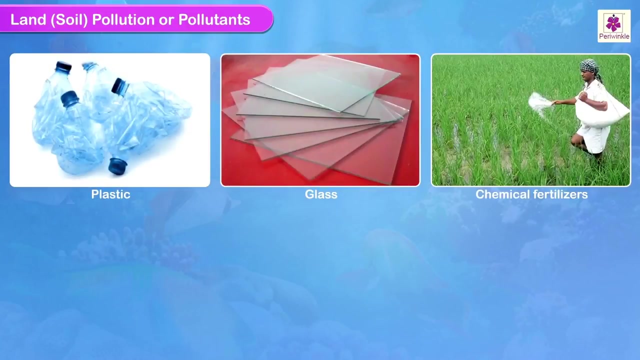 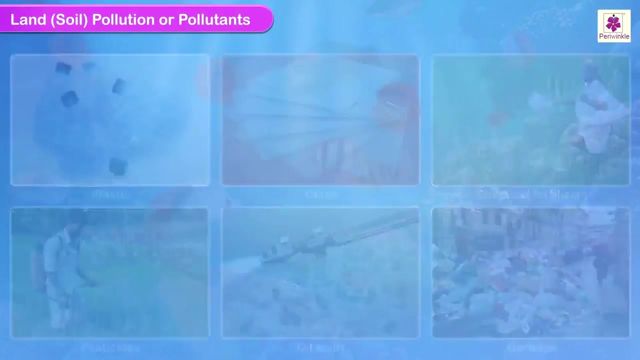 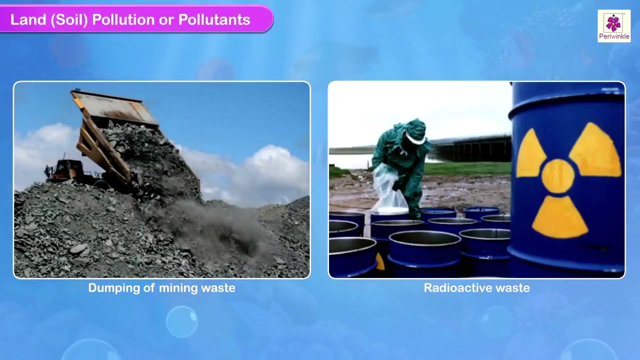 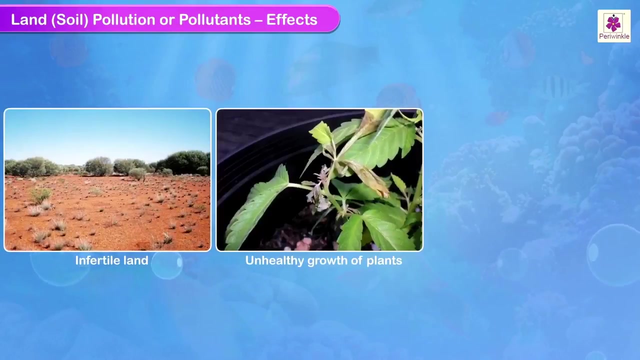 Land, ie soil pollution or pollutants, Plastic, glass, chemical fertilizers, pesticides, oil spills, garbage, Dumping of mining waste and radioactive waste. The most dangerous one are some land pollutants. Effects In fertile land, unhealthy growth of plants, low farm yields are some of the effects of land pollution. 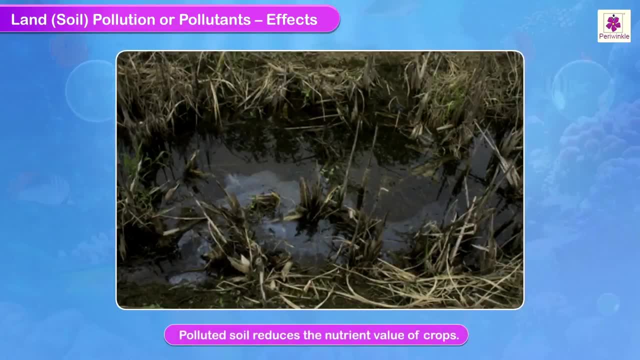 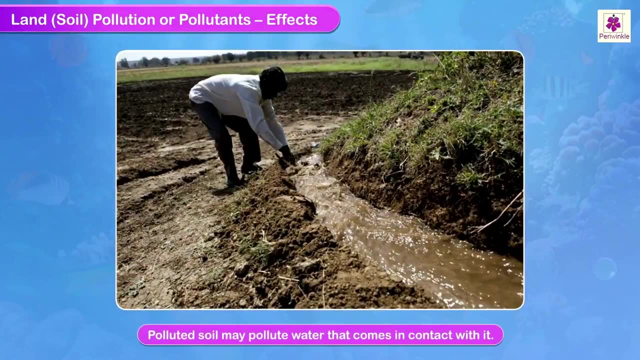 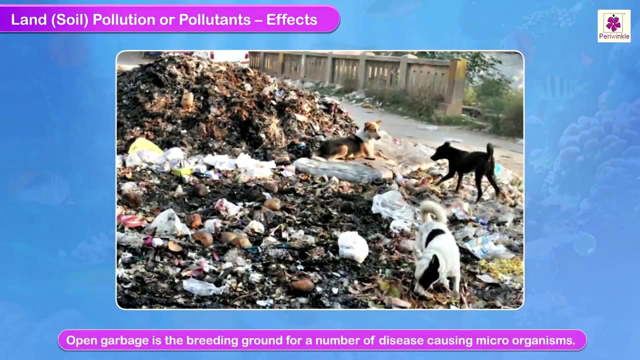 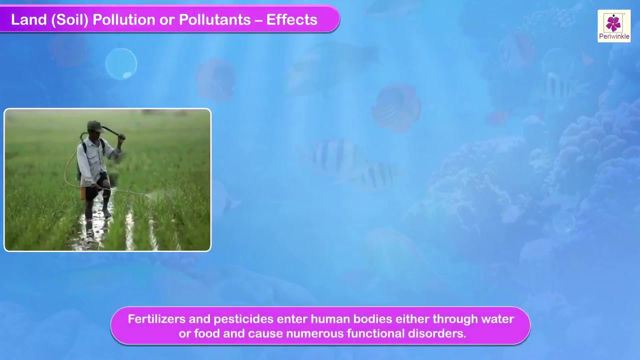 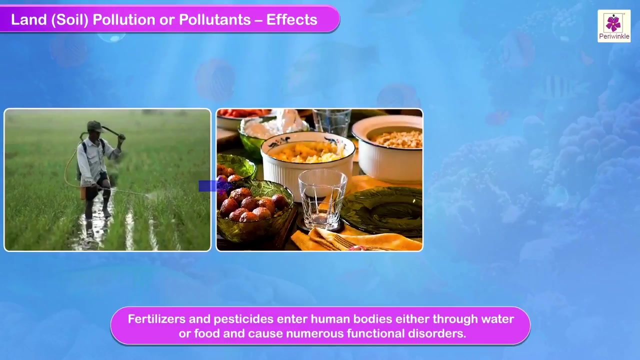 Polluted soil reduces the nutrient value of crops. Polluted soil may pollute water that comes in contact with it. Open garbage is the breeding ground for a number of disease-causing microorganisms. Fertilizers and pesticides enter human bodies either through water or food and cause numerous functional disorders. 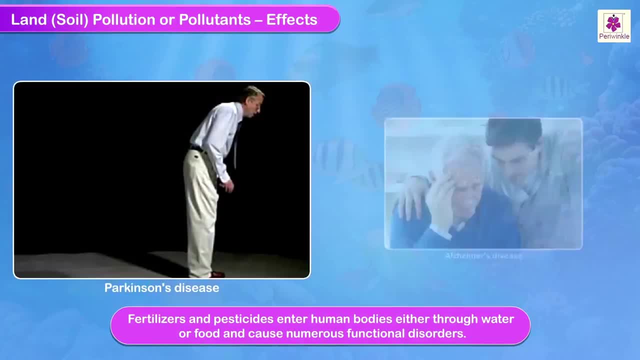 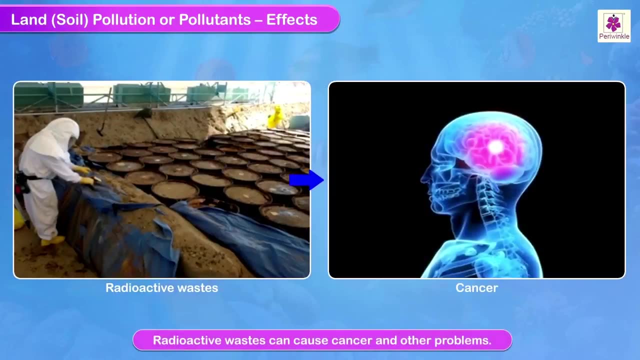 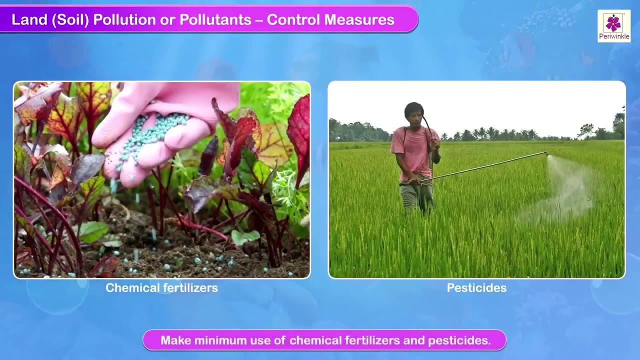 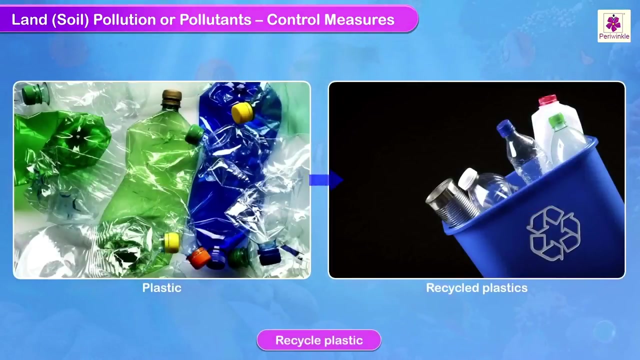 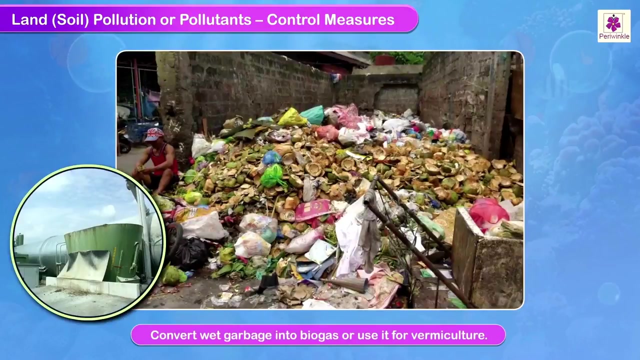 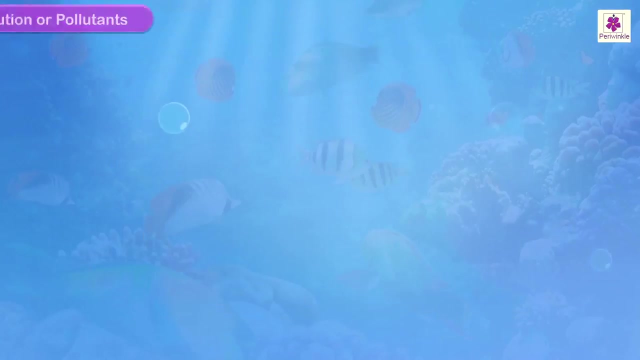 such as Parkinson's or Alzheimer's disease. Radioactive wastes can cause cancers and other problems. Control measures: Make minimum use of chemical fertilizers and pesticides. Recycle plastics. Convert wet garbage into biosecurity biogas or use it for vermiculture. regulate dumping of mining wastes. noise. 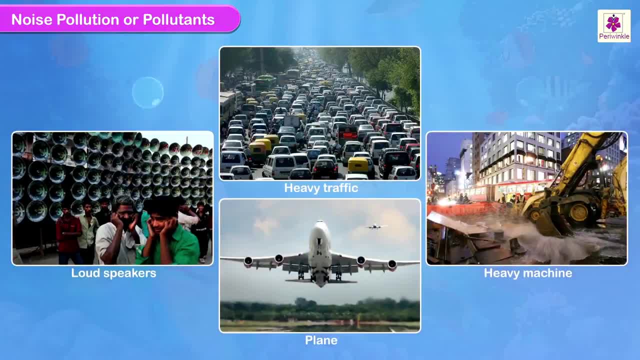 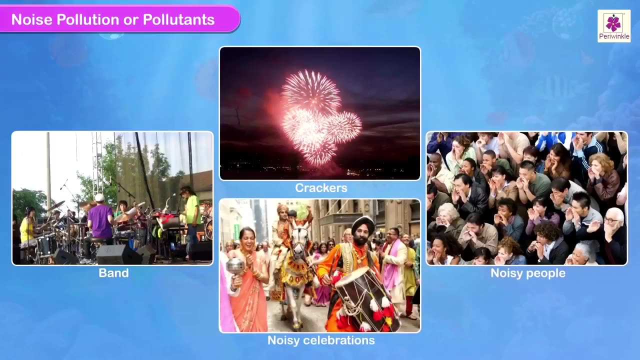 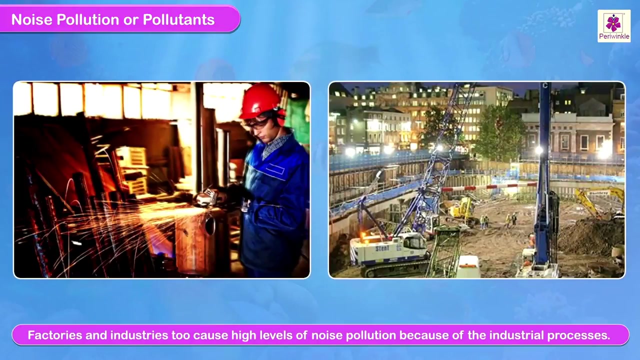 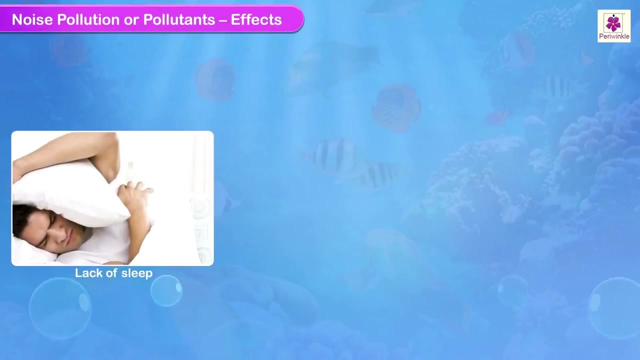 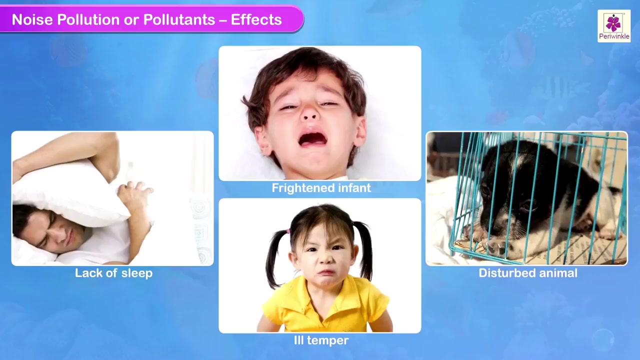 pollution or pollutants noise, especially from loudspeakers, heavy traffic, heavy machines, planes, bands, crackers, noisy people and noisy celebrations are some of the common sources of noise pollution. factories and industries to cause high levels of noise pollution because of the industrial processes effects, disturbed sleep or lack of sleep, frightened infants, disturbed animals, ill. 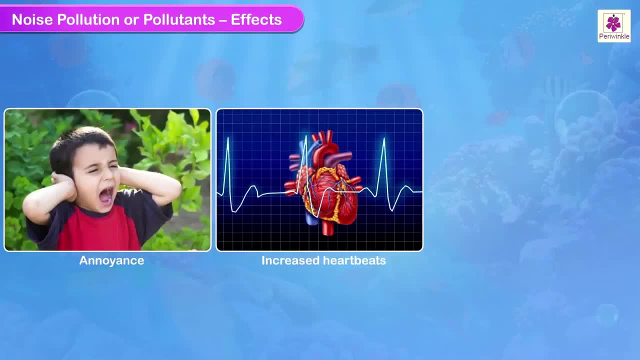 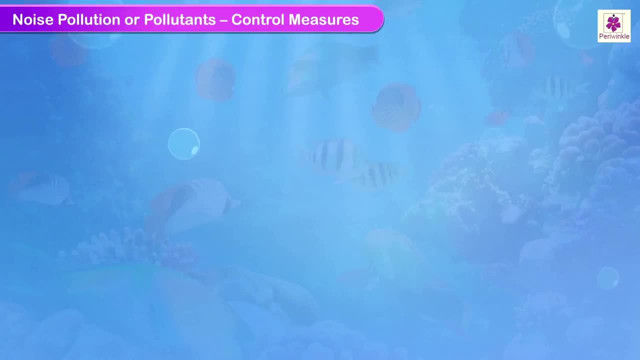 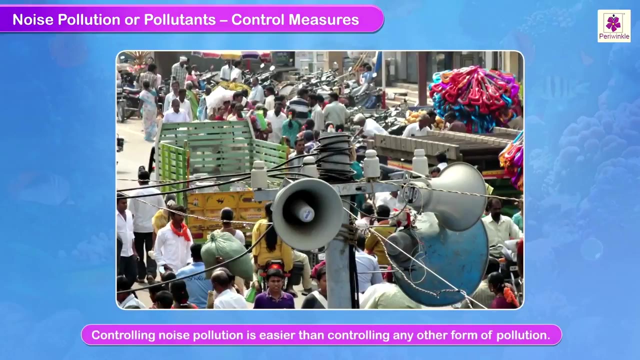 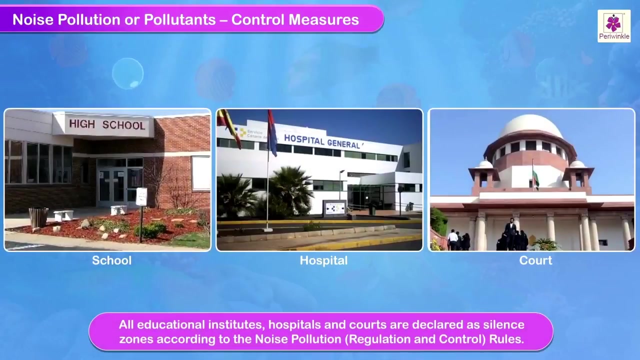 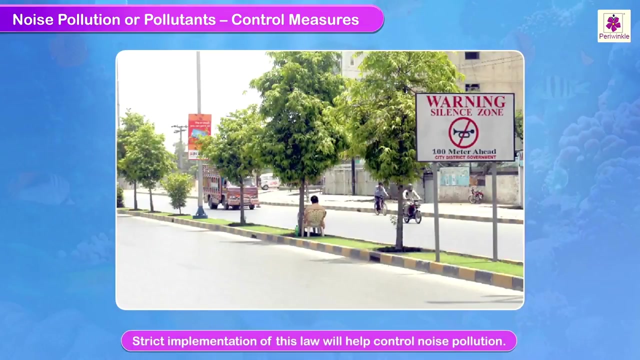 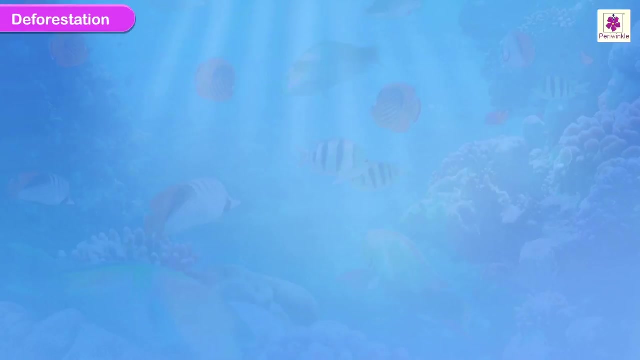 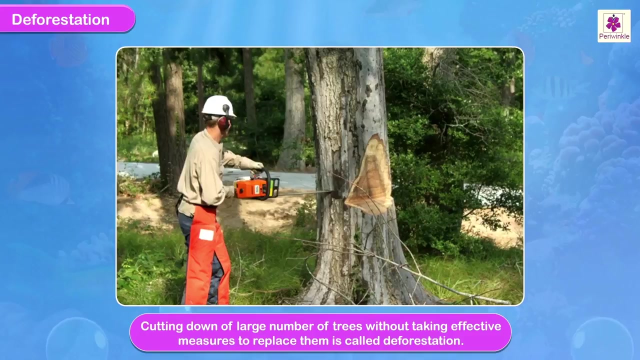 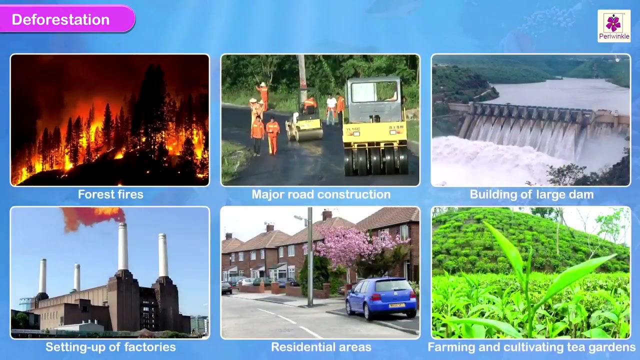 temper, annoyance, increased heartbeats, deafness are effects of noise pollution control measures. controlling noise pollution is easier than controlling any other form of pollution. all, not we. first this room is necessary. legislation, including have taken effective management measures to replace them is called deforestation. Forests are destroyed due to forest fires, major road construction activities, building. 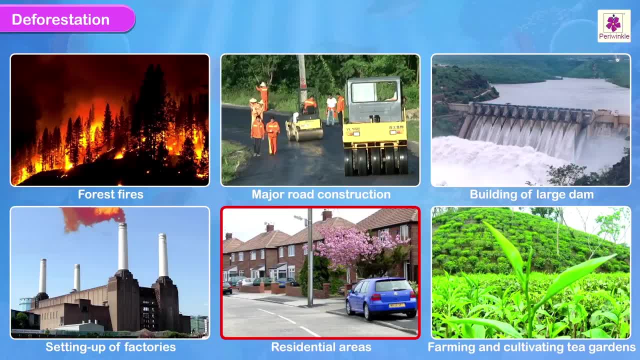 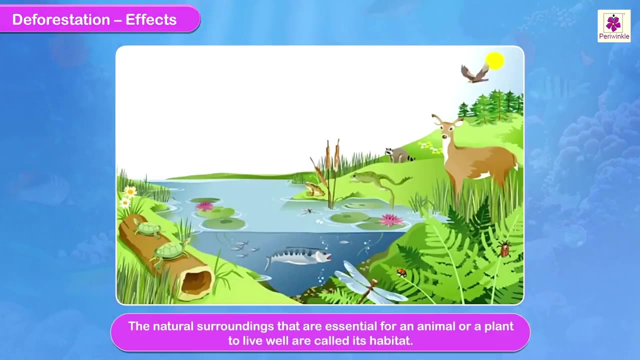 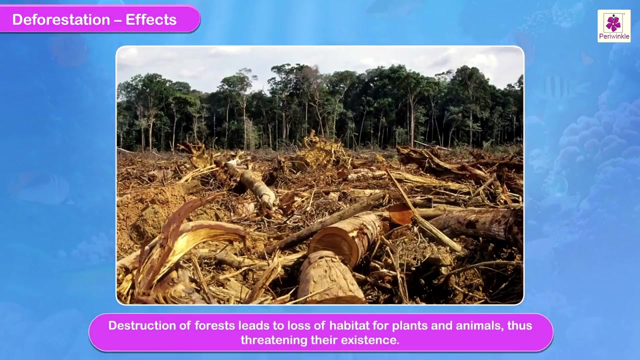 of large dams, setting up of factories, residential areas, farming and cultivating, tea gardens, etc. Effects. The natural surroundings that are essential for an animal or a plant to live well are called its habitat. Destruction of forests leads to loss of habitat for plants and animals, thus threatening their 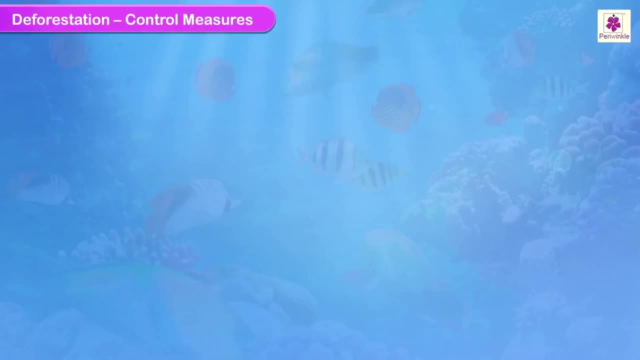 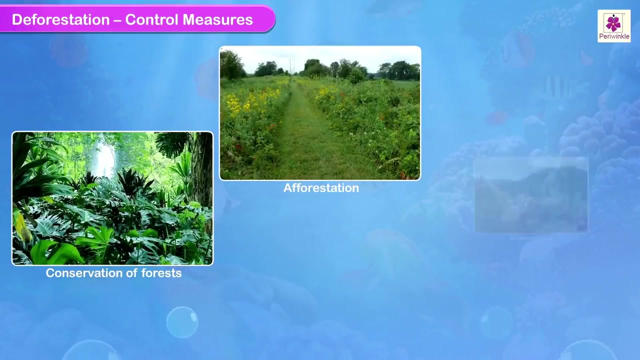 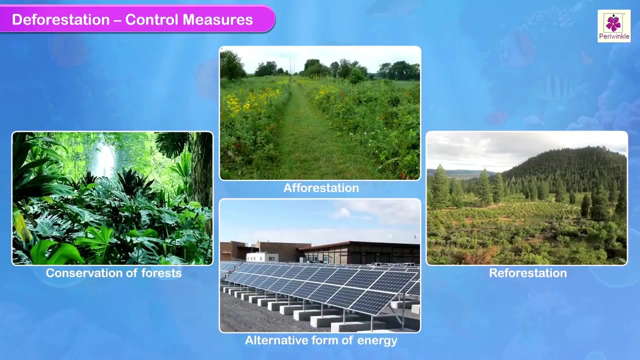 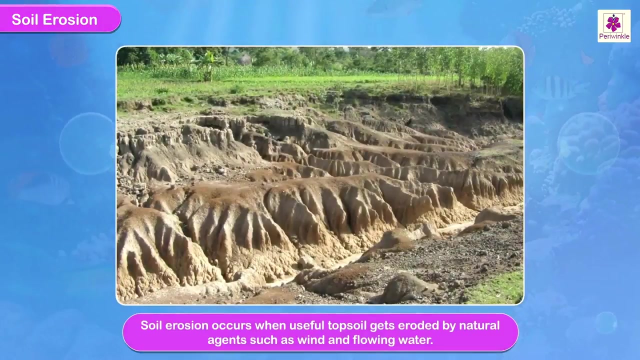 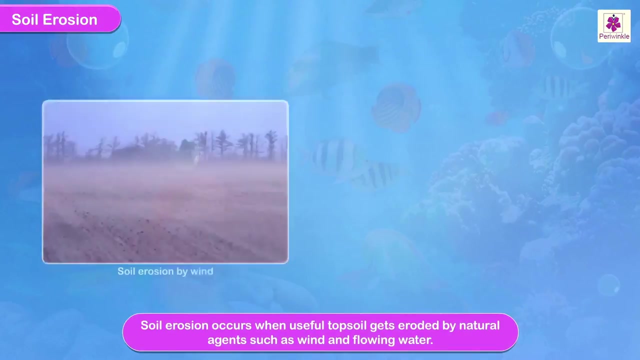 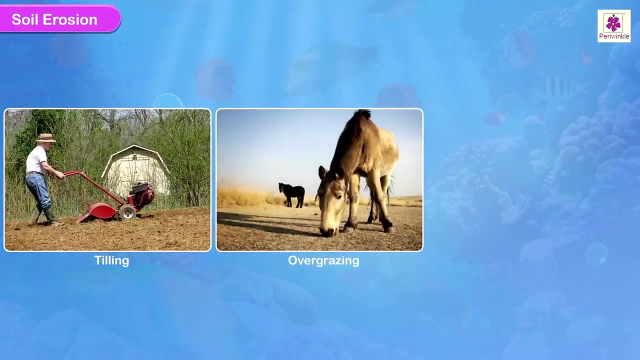 existence Control measures. Conservation of forests, afforestation, reforestation, use of alternative forms of energy are some control measures. Soil erosion: Soil erosion occurs when useful topsoil gets eroded by natural agents such as wind and flowing water. If the 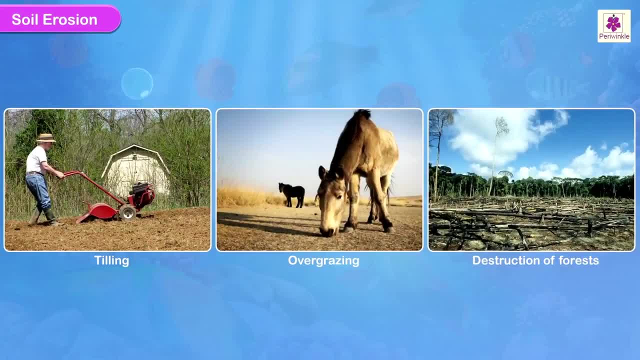 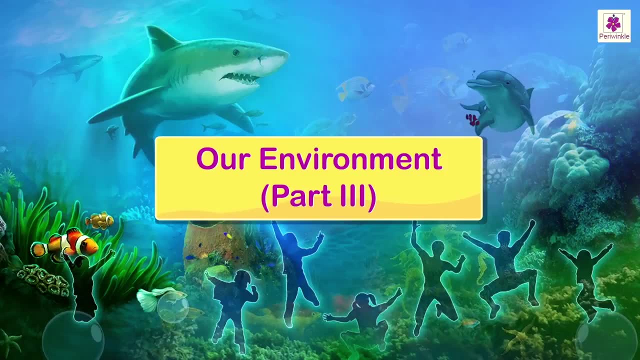 topsoil is eroded too quickly, then advised of. here are three common sources of soil erosion problems, and often are minimal. in really simple wordsEMERGENCY PROGRAMS. union dressed without DAMS Reusable ‬. Nor greet Or Soil has plusx. 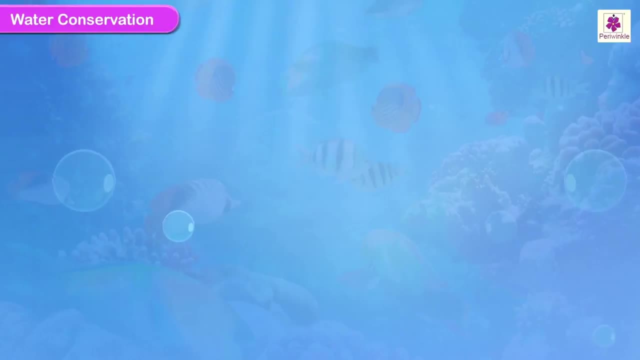 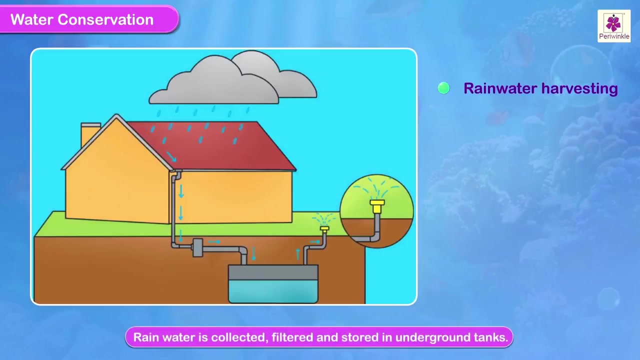 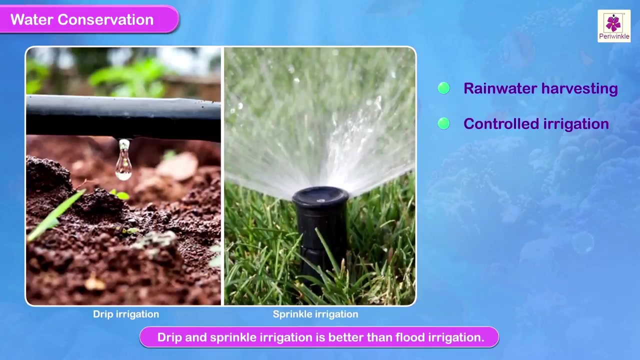 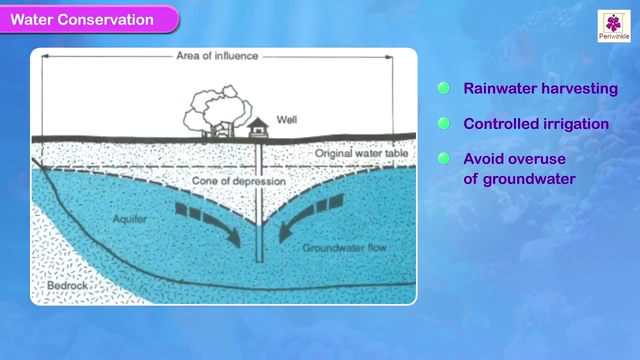 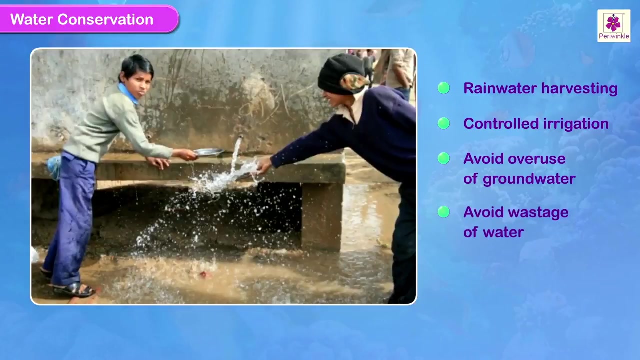 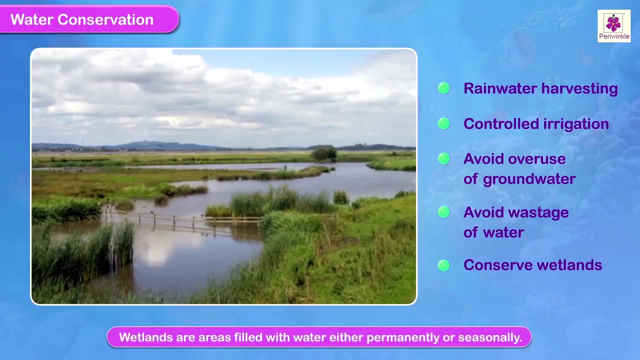 socially. Maybe Bass Is Water. Water harvesting. rain water is collected, filtered and stored in underground tanks. controlled irrigation- drip and sprinkle irrigation is better than flood irrigation. avoid overuse of groundwater. if large amounts of groundwater is withdrawn, the water table falls drastically. avoid wastage of water. conserve wetlands. wetlands are areas filled with water, either permanently or 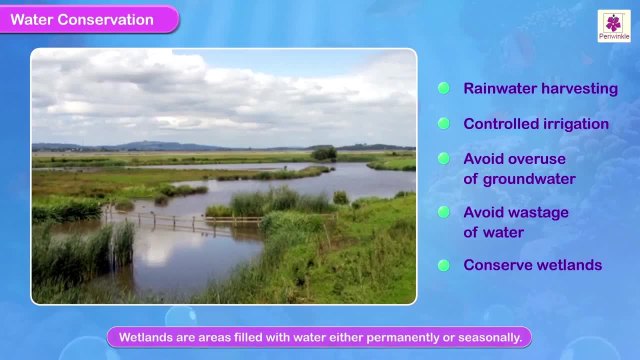 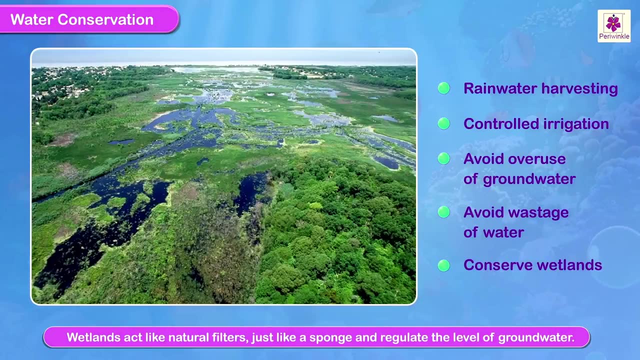 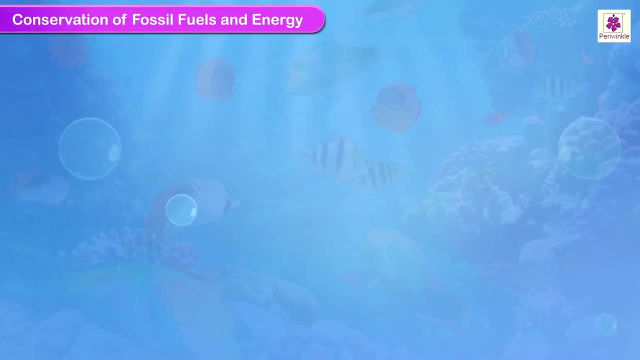 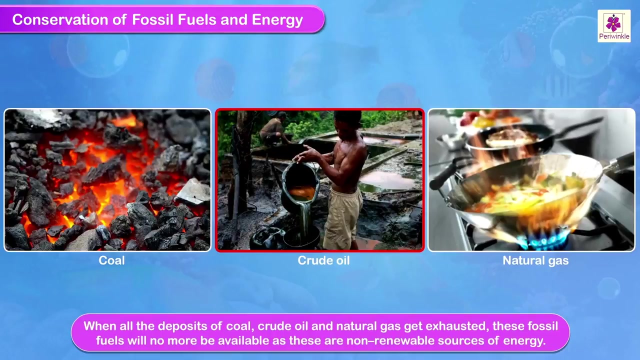 seasonally, wetlands act like natural filters, just like a sponge, and thus regulate the level of water that is stored in the tank of groundwater. conservation of fossil fuels and energy. when all the deposits of coal, crude oil and natural gas get exhausted, these fossil fuels will no 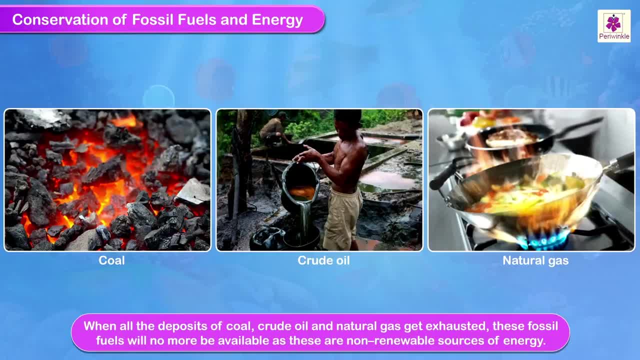 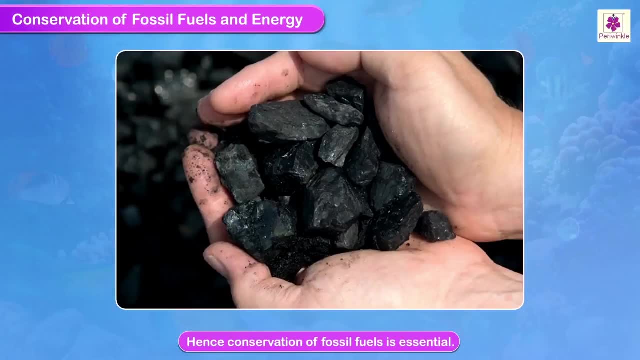 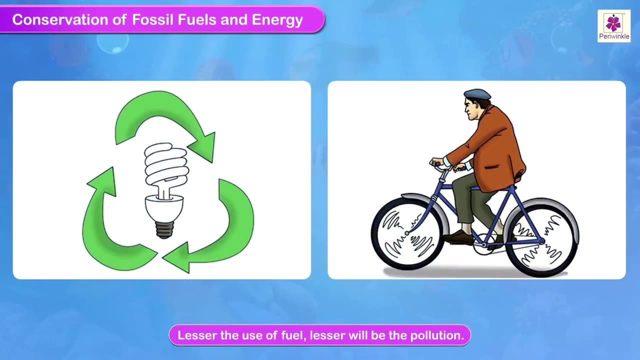 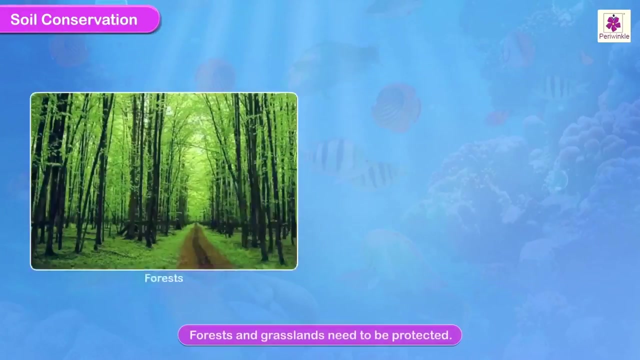 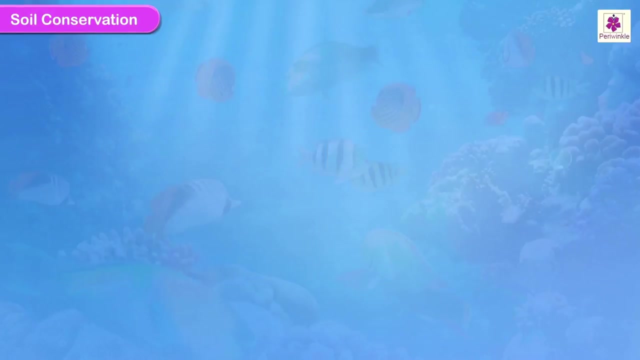 more be available, as these are non-renewable sources of energy. hence their conservation is essential. moreover, lesser the use of fuel, lesser will be the pollution. Sean conservation, forest and grasslands need to be protected. afforestation, bunding agriculture, contour farming, prevention of over grazing are some ways to control the selection of areas in soil conservation. 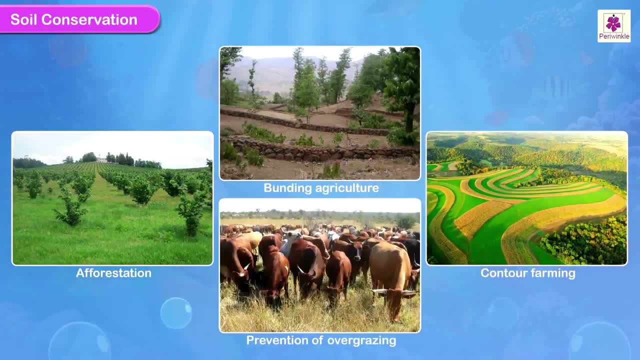 соответ이다. con24 is a croisance Bible in settle and finance its research in the world. as그 danim往long tarot. reading of the author: 17 Letter inscribed at mediathek Maori that the definition of grave不過 crisis is theRead anoats on slope in kiatalecta. ultimately, historical setting: 653: know here this is a real會. 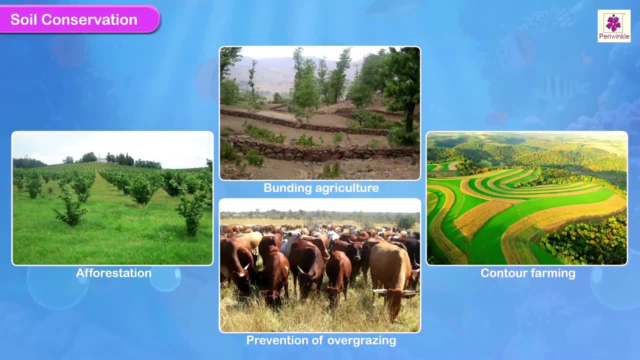 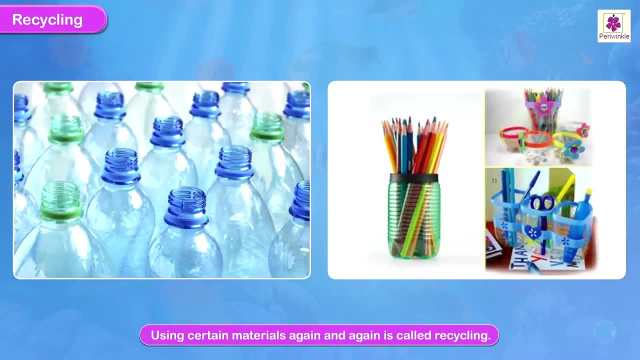 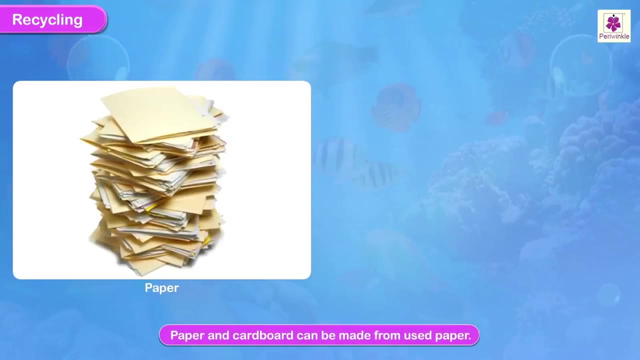 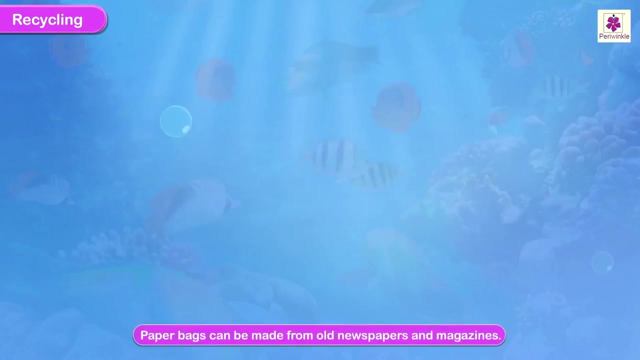 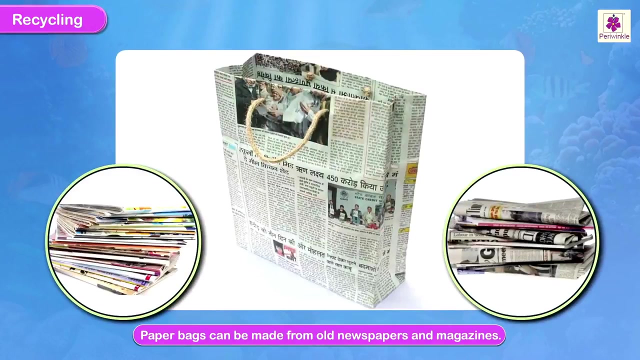 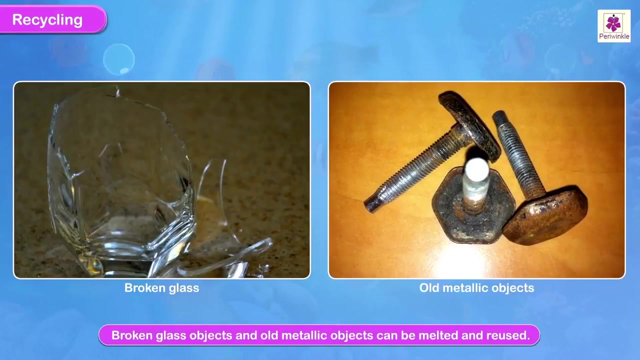 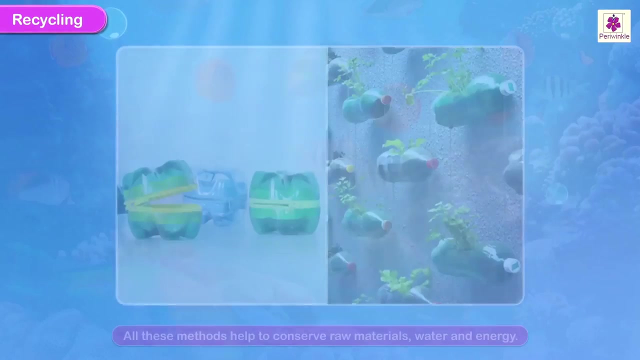 ways to prevent soil erosion. Recycling, Using certain materials again and again, is called recycling. Paper and cardboard can be made from used paper. Paper bags can be made from old newspapers and magazines- ie reusing Broken glass objects. and old metallic objects can be melted and reused. 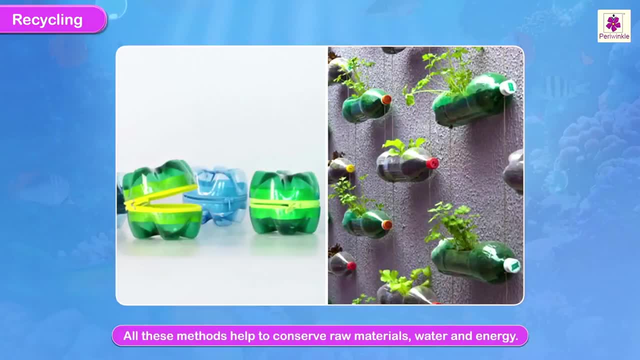 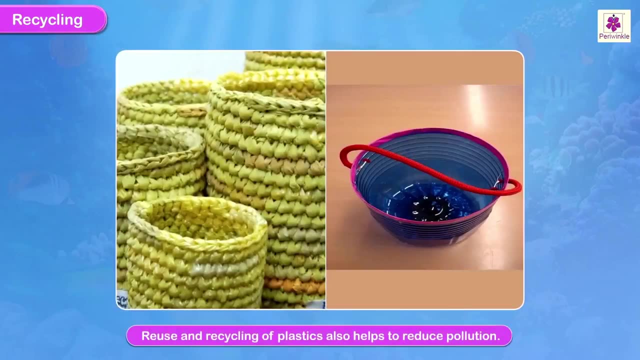 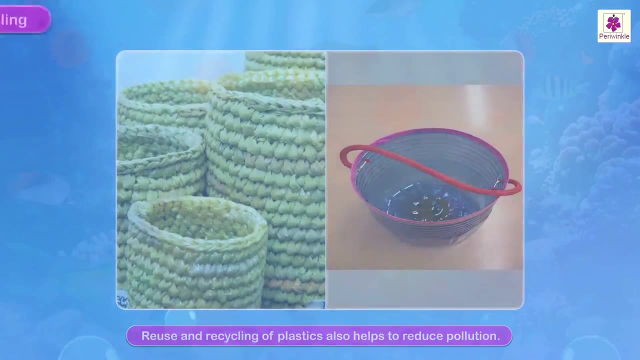 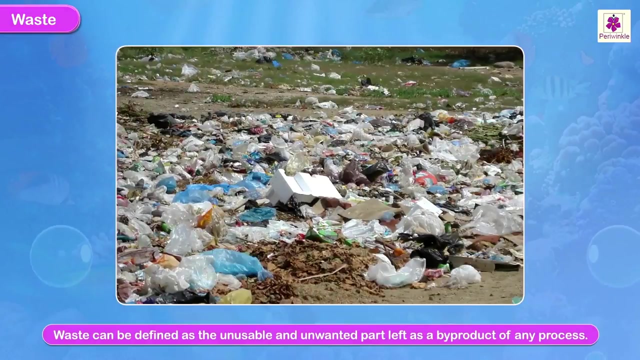 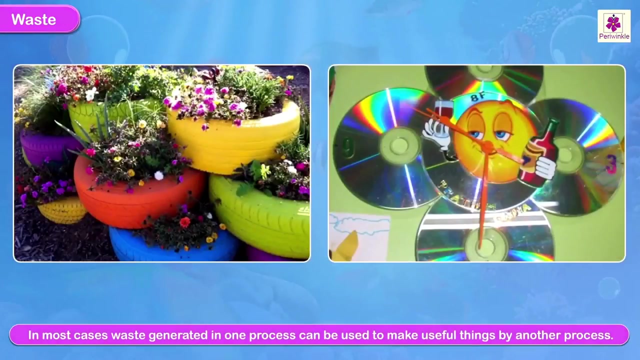 All these methods help to conserve raw materials, water and energy. Recycling, Reuse and recycling of plastics also help to reduce pollution Waste- Waste can be defined as the unusable and unwanted part left as a byproduct of any process, In most cases, waste generated in one process. 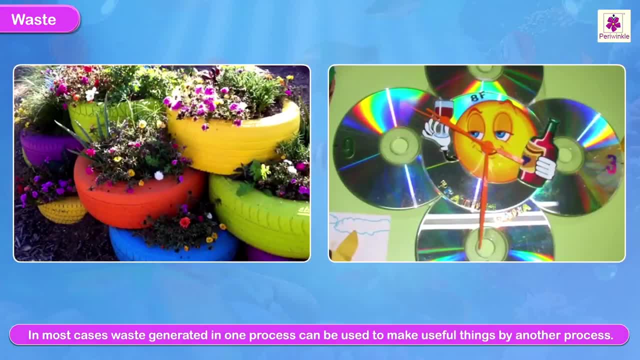 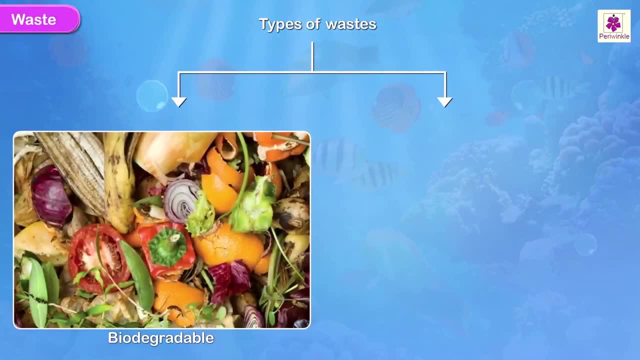 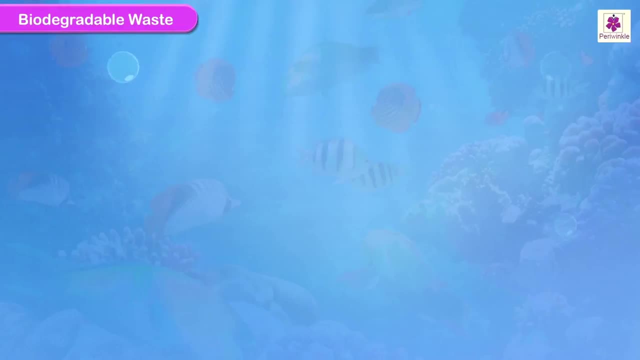 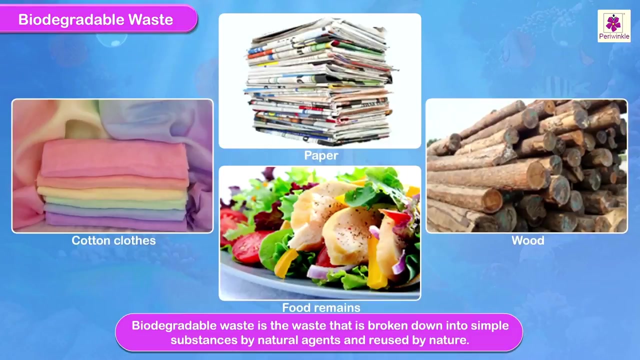 can be used to make useful things by another process. There are two types of wastes: biodegradable and non-biodegradable. Biodegradable Waste- Biodegradable waste- is the waste that is broken down into simple substances by natural agents and reused by nature. 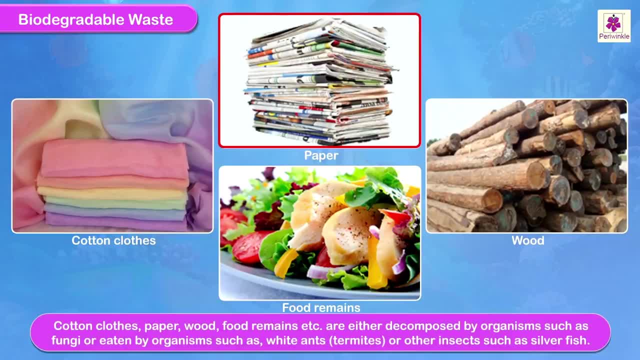 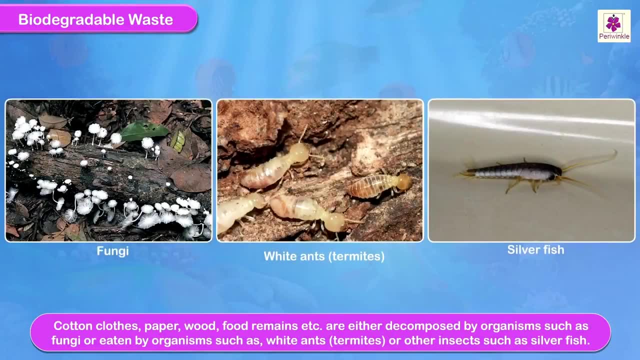 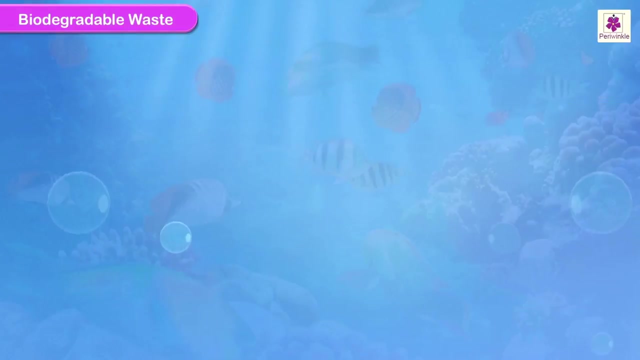 For example, cotton, clothes, paper, wood, food remains, etc. are either decomposed by organisms such as fungi or eaten by organisms such as white ants, ie, termites or other insects such as silverfish. Biodegradable Wastes. Biodegradable wastes are regularly used up or reused. 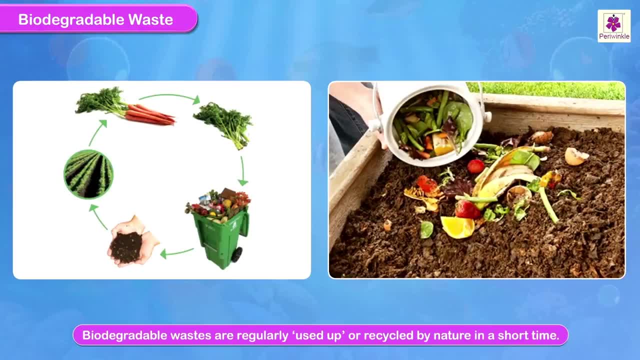 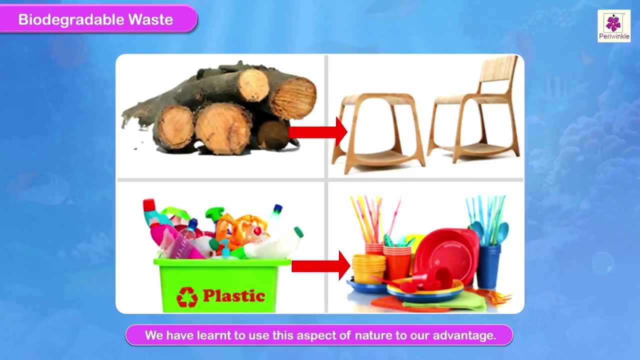 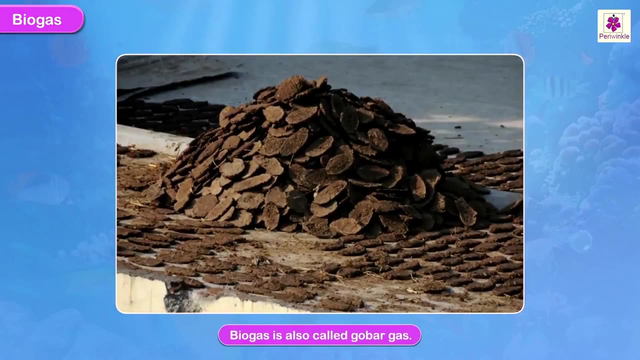 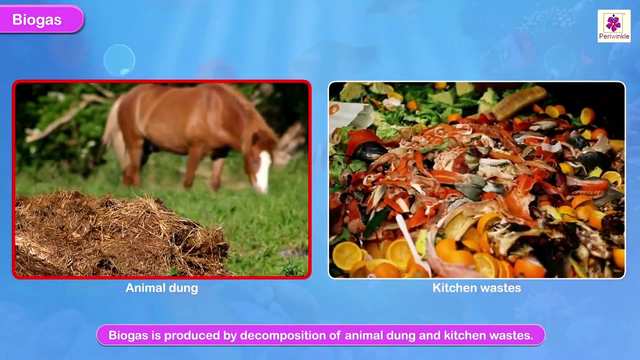 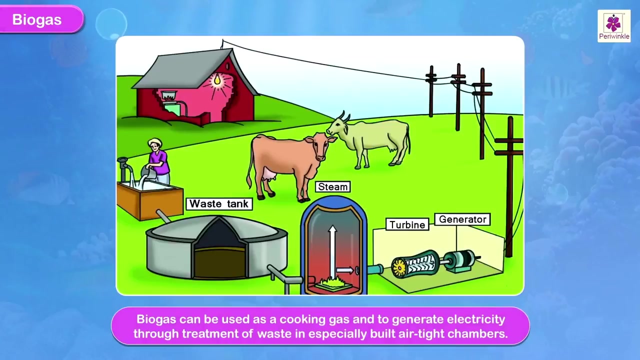 They are recycled by nature in a short time. We have learned to use this aspect of nature to our advantage. Biogas- It is also called gobar gas. It is produced by decomposition of animal dung and kitchen wastes. Biogas can be used as a cooking gas and to generate electricity through treatment of waste in especially built, airtight chambers. 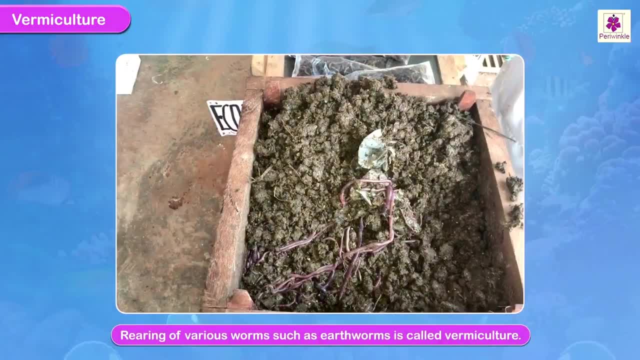 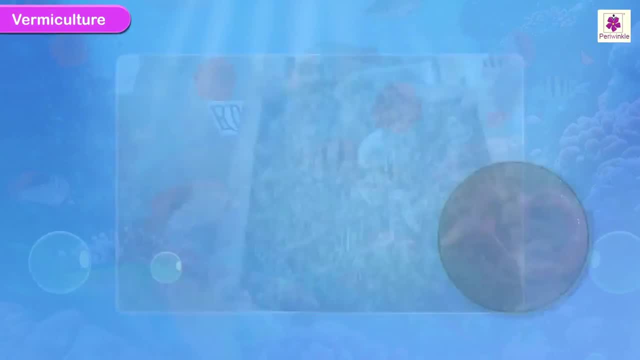 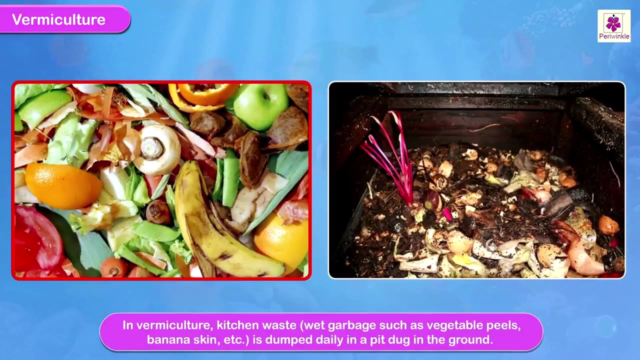 Vermiculture Rearing of various worms such as earthworms is called vermiculture Kitchen Waste. In vermiculture kitchen waste- that is, wet garbage such as vegetable peals, banana skin etc. is dumped daily in a pit dug in the ground. 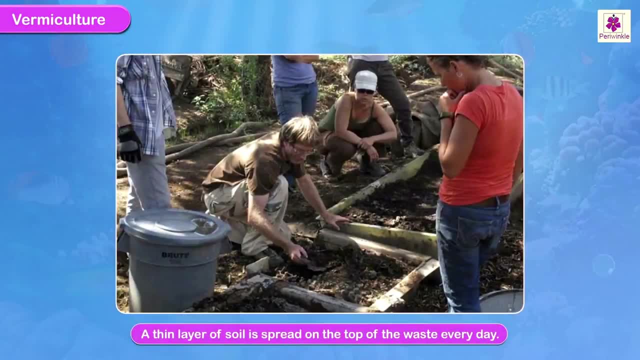 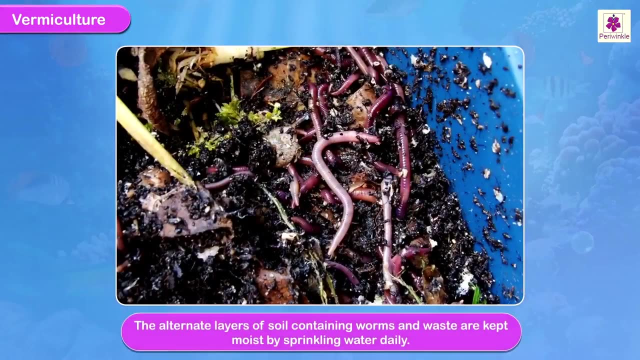 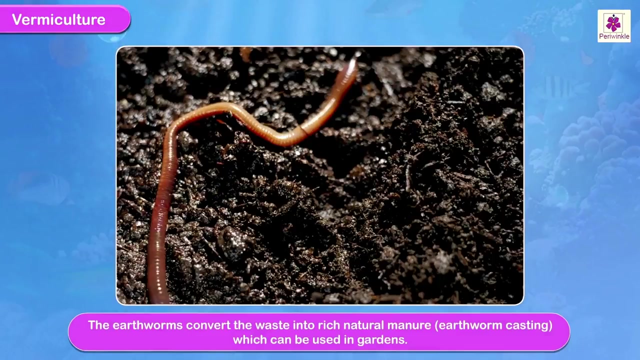 believed to be your part of your environment. and a thin layer of soil is spread on top of the waste every day Masks- The alternate layers of soil containing worms and waste, are kept moist, sprinkling water daily. in a few days, the earthworms convert the waste into rich. 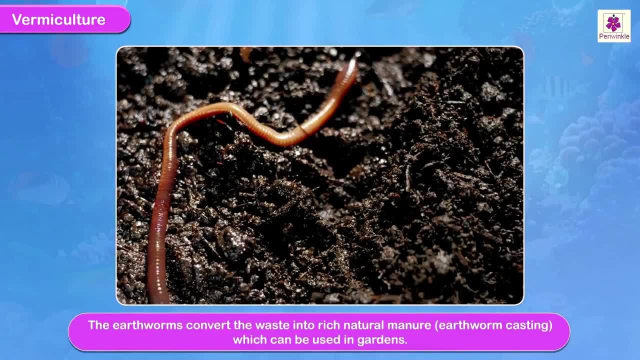 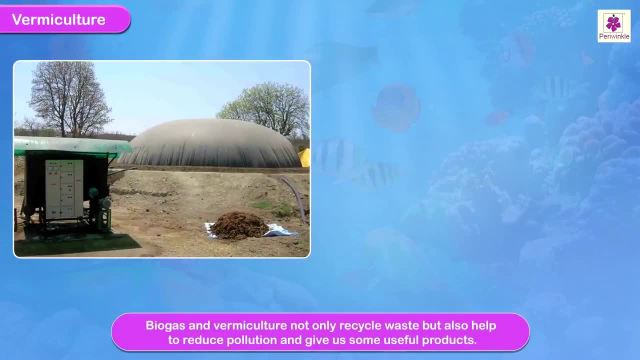 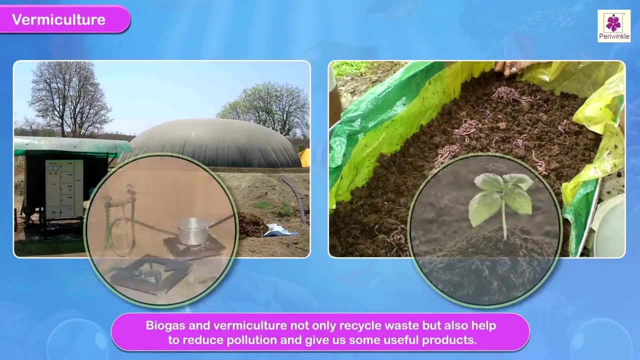 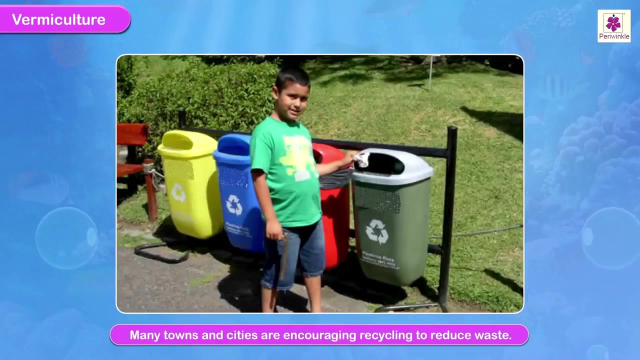 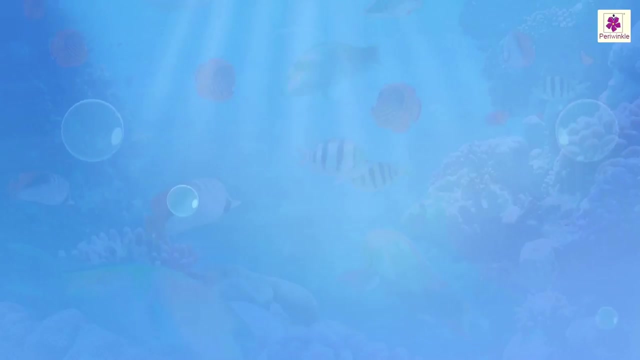 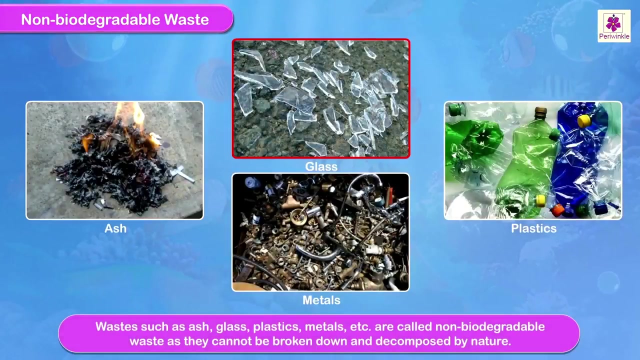 natural manure, that is, earthworm casting, which can be used in gardens. biogas and vermiculture not only recycle waste, but also help to reduce pollution and give us some useful products. many towns and cities are encouraging recycling to reduce waste. non bio-degradable based waste such as ash, glass, plastics, metals.